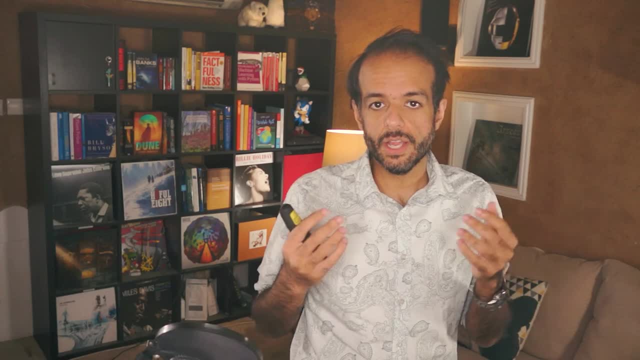 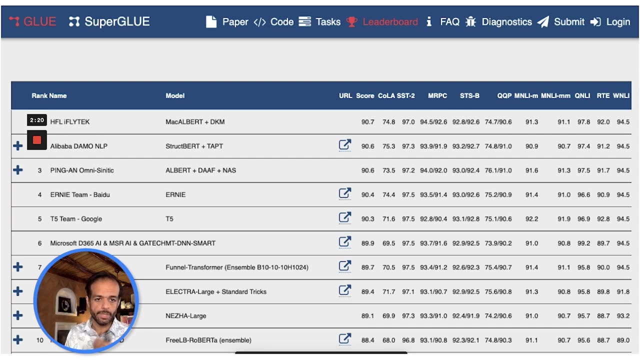 basically is a type of machine learning model. It's an architecture of neural networks. Since then we've been looking at it for decades and we're very excited to have it. So the variants of the transformer, namely a variant called BERT that builds on top of the transformer, has grown to. 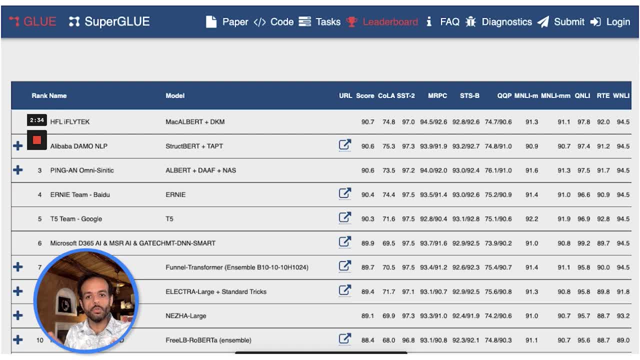 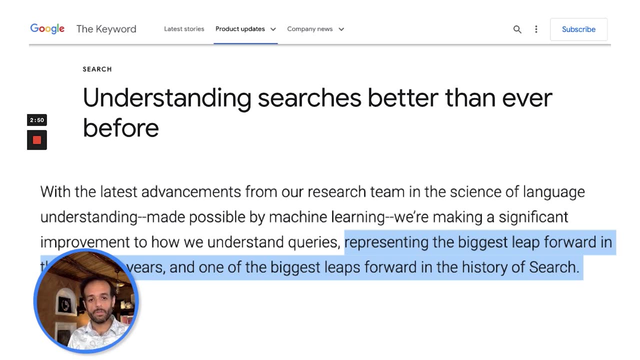 dominate the models of natural language processing in various tasks. These are some leaderboards that researchers use to rank and rate models, And the top scoring models from this snapshot are all based on BERT, which is based on the transformer- transformer-based models to Google Search. 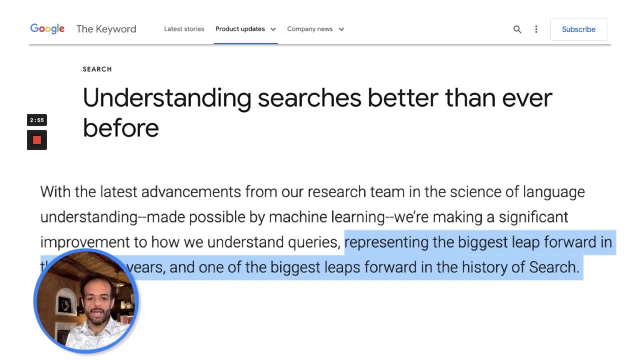 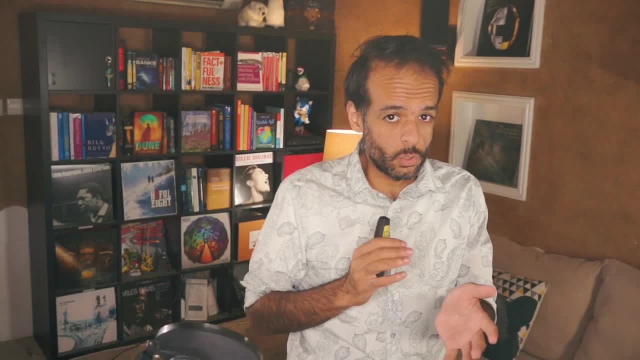 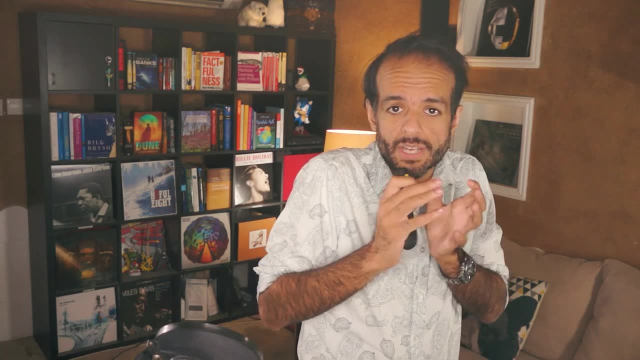 They've been using them to empower Google Search and they call it one of the biggest leaps forward in the history of search. So this is important stuff Now, over the last two weeks, we have developments that extend the value of transformers beyond just natural language processing. 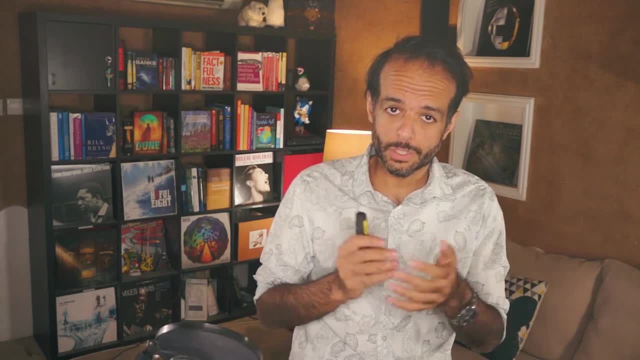 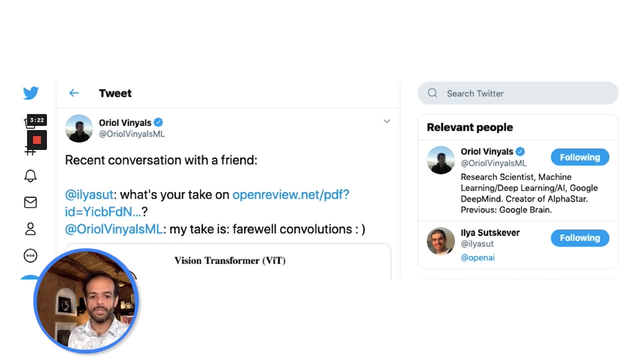 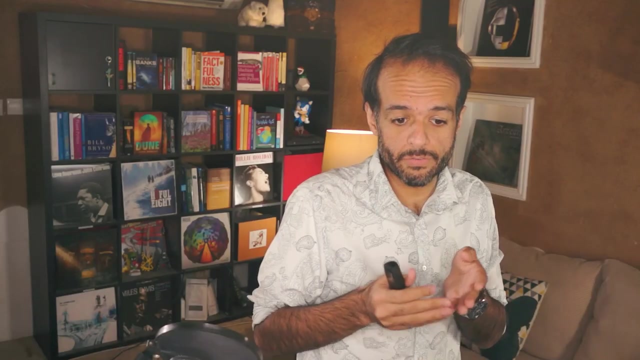 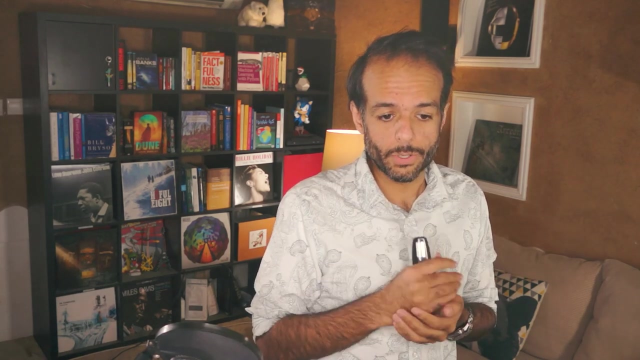 And so this is a conversation between two senior AI and ML researchers, and Oriol is in DeepMind and Ilya is the head scientist in OpenAI And based on this paper on vision transformers that applied transformers to computer vision, and Oriol thinks that it's farewell to convolutions. 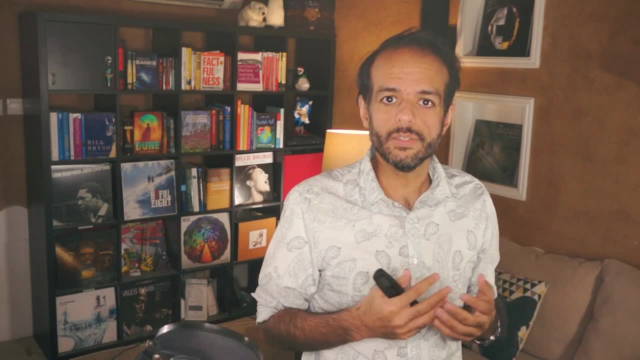 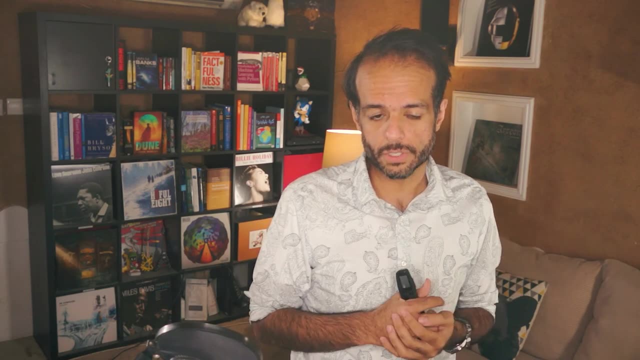 And so deep learning in computer vision has been dominated by convolutional neural networks that have been producing the best deep learning models in computer networks, And that's what we're seeing in computer vision. But right now, starting from a few weeks ago, we're starting to see transformer-based models. 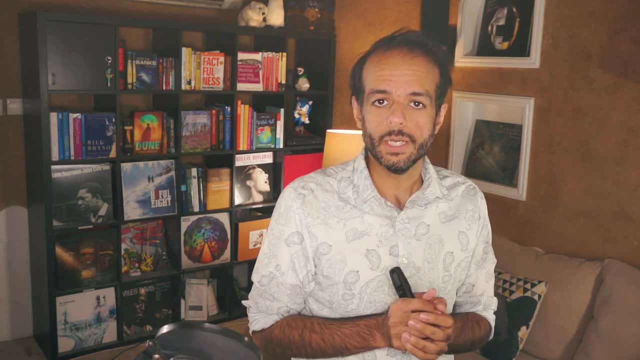 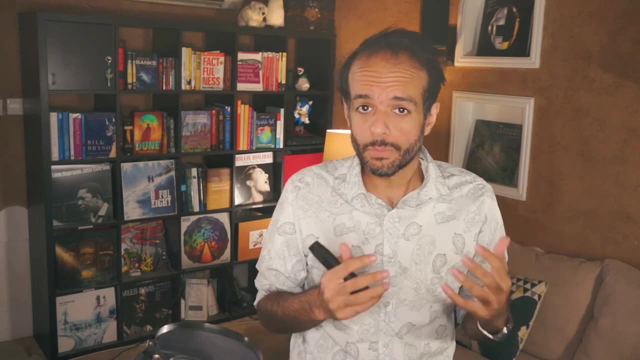 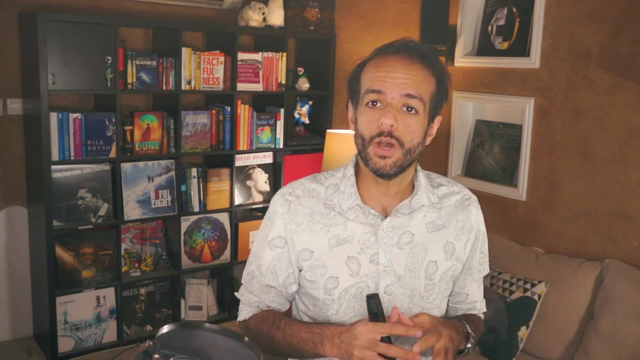 that seem to be doing results that are really impressive in computer vision. So transformers are getting more and more important. So not just in natural language processing, but now it's going to extend its surface area, I guess, to other areas of deep learning beyond just language. 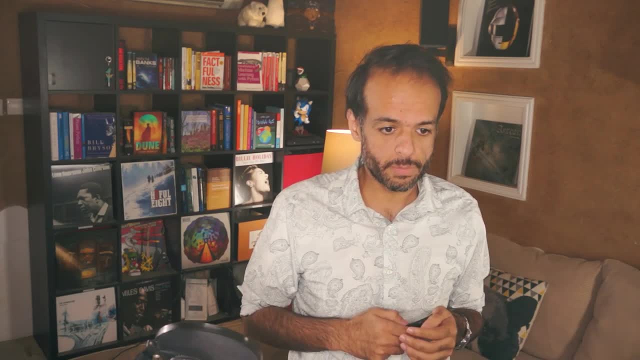 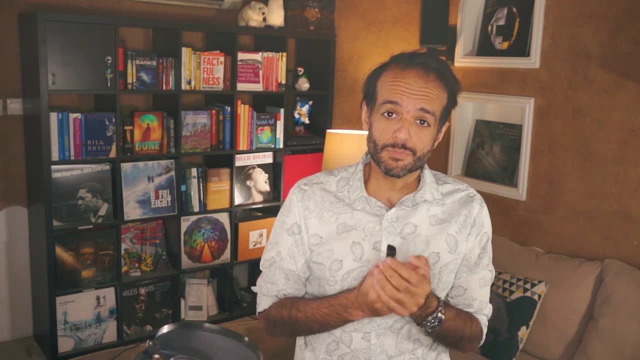 And so it's never too late. It's never too late to learn about them. They're fascinating. They keep getting more and more important. as an architect Now, I've written this blog post before, called the Illustrated Transformer, I think two years ago. 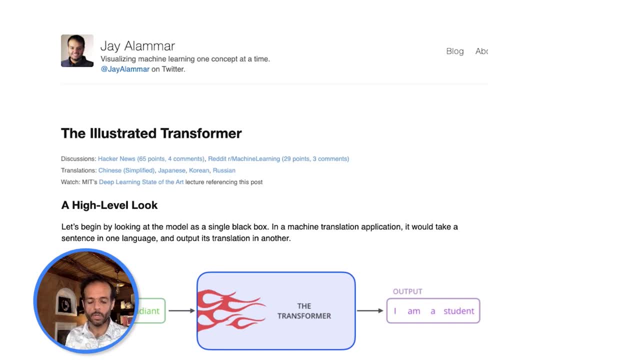 About a million page views, I believe, of people who were able to learn about transformers based on just some of the visualizations, some of the ideas that I When I read the paper and went over the code. that's how I understood the transformers. 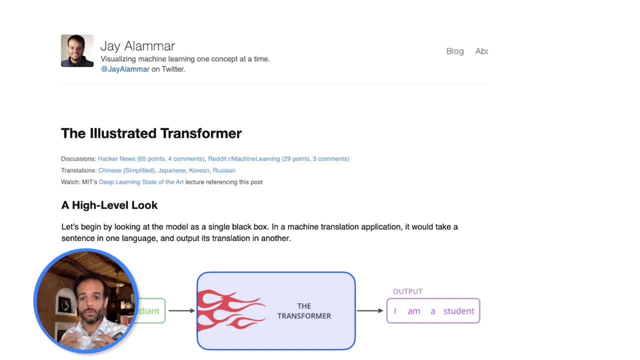 and I illustrated it in this series, And so in this video we'll describe the transformer again, And if you want any more details than the things that we'll be discussing here, you can revert back to my blog. You can just search for the Illustrated Transformer. 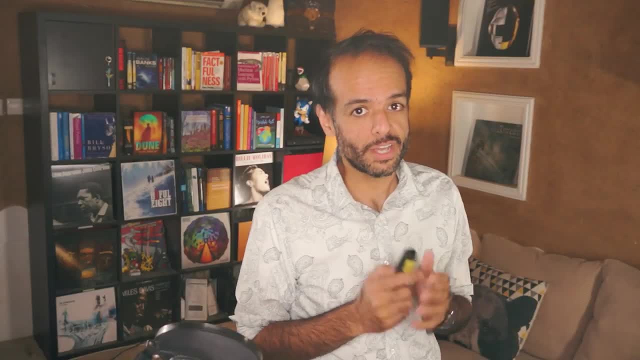 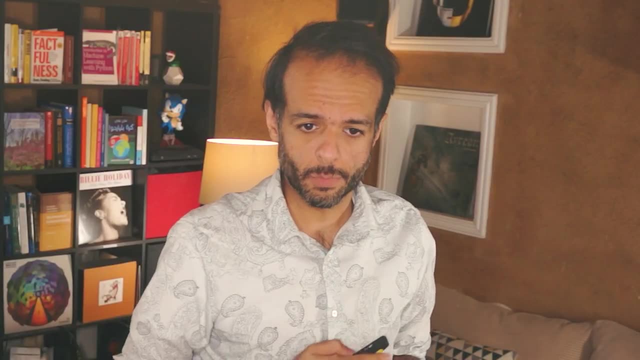 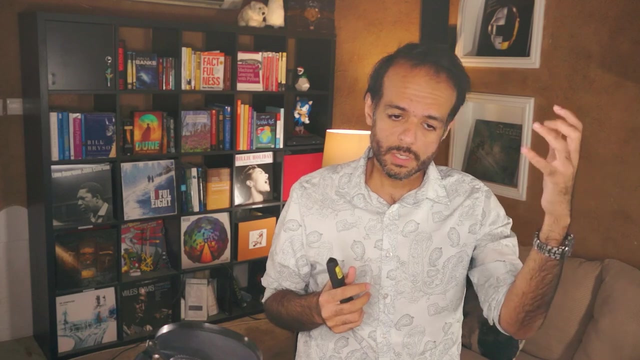 and you'll find a lot more details. So let's get right into it. Let's talk a little bit about the architecture of a trained model. We can think about a transformer as a black box, a blue box in this case. that takes a sequence. 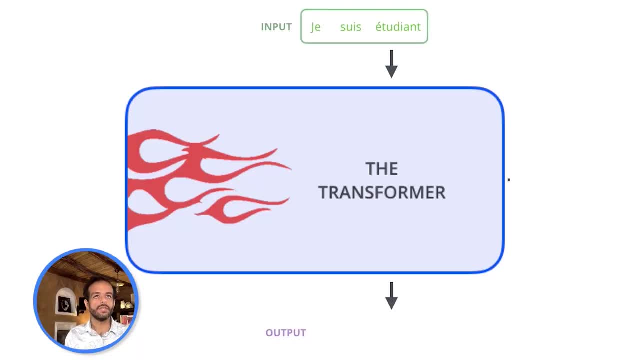 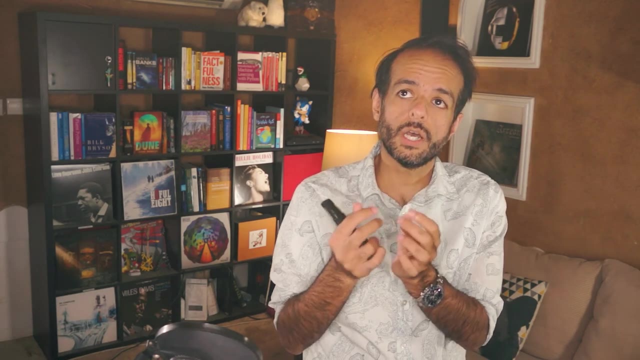 let's say, three-word phrase in French and outputs it as an English phrase. So it outputs- I am a student if it's given that French sentence- And that's the example from the initial paper, because the initial paper talked about machine translation models. 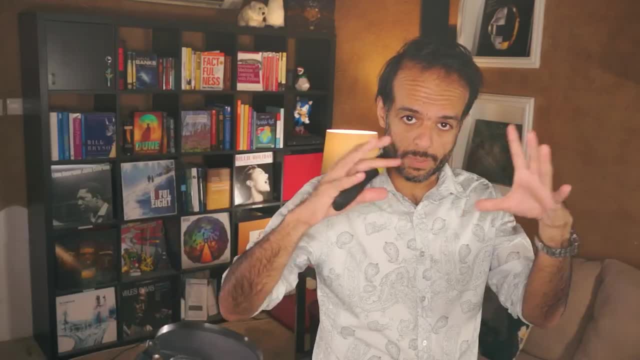 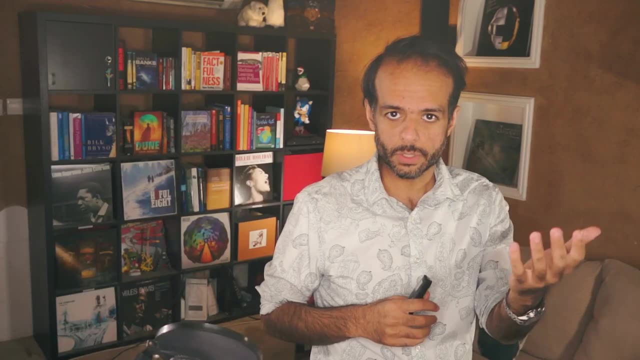 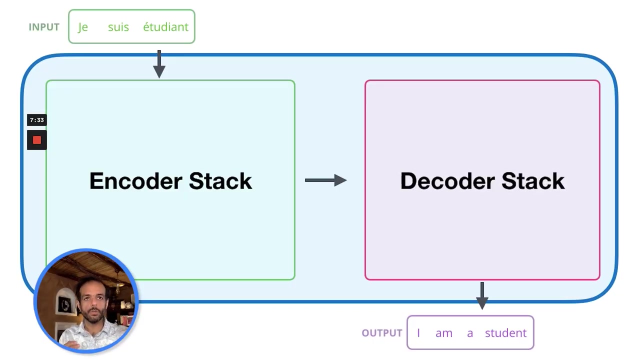 We broke down that general black box into two smaller components, two smaller black boxes, let's say inside of it. One is an encoder stack, so the input goes to the encoder stack and then outputs some of its processing results to a decoder stack. 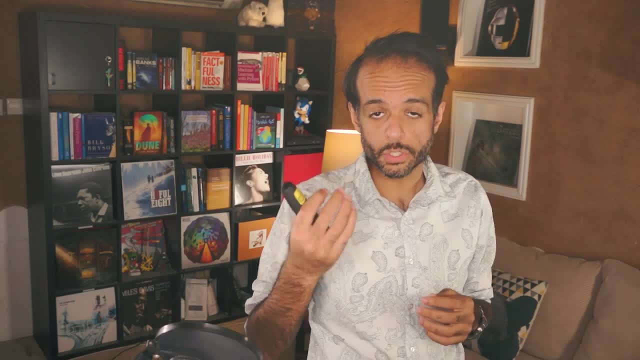 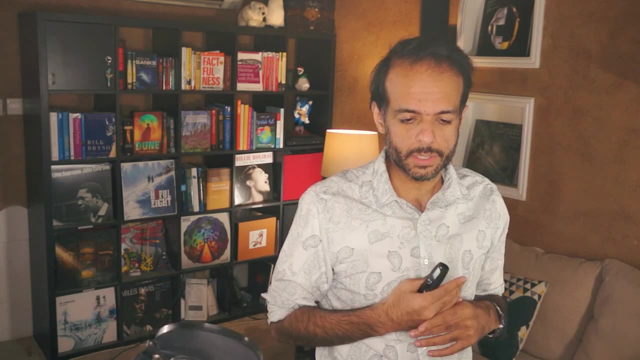 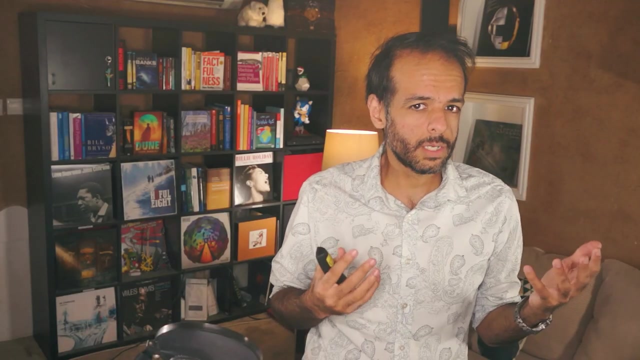 and the decoder stack outputs. the output words or tokens. And then we mentioned that the stacks, each of them, is composed of layers, six layers each. in the initial transformer of encoders and decoders, These grew to be called transformer blocks. The initial paper doesn't call them that. 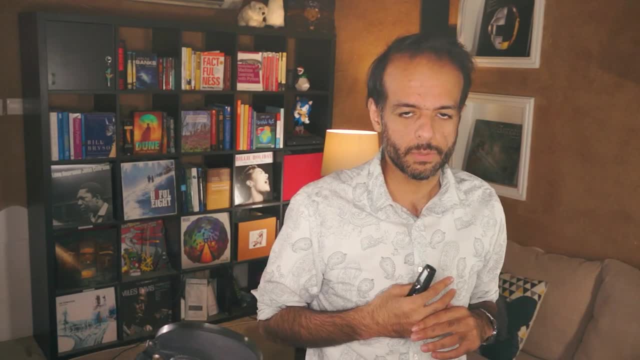 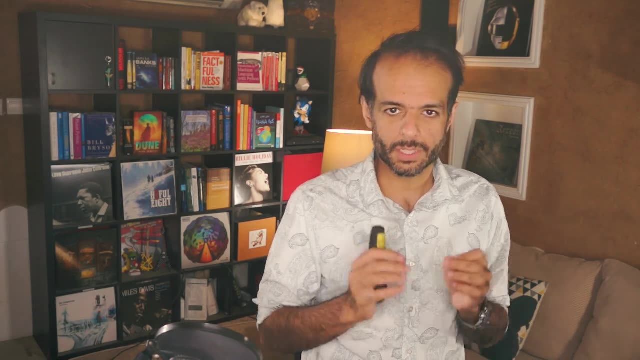 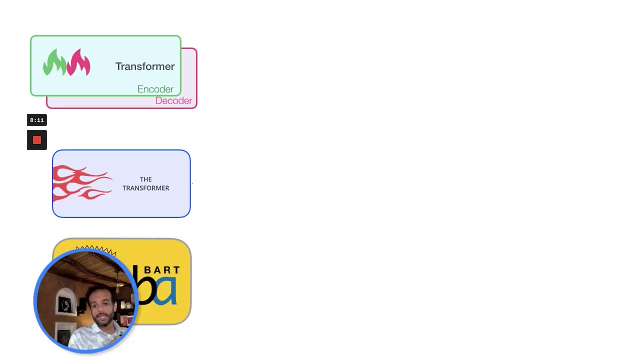 but later papers, I believe, start calling it that. So transformer encoder blocks and transformer decoder blocks are the building blocks of transformers. Now, the initial transformer is an encoder-decoder model, as we've seen, And that is still the case with models like BART. 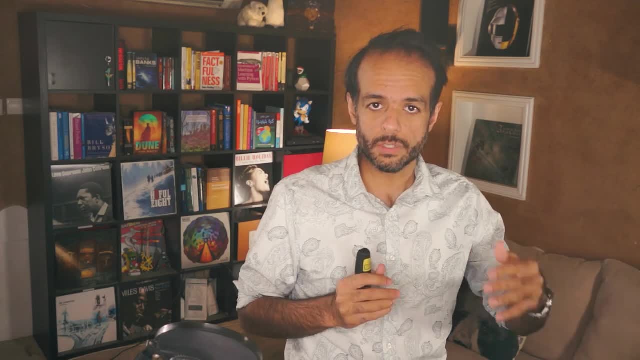 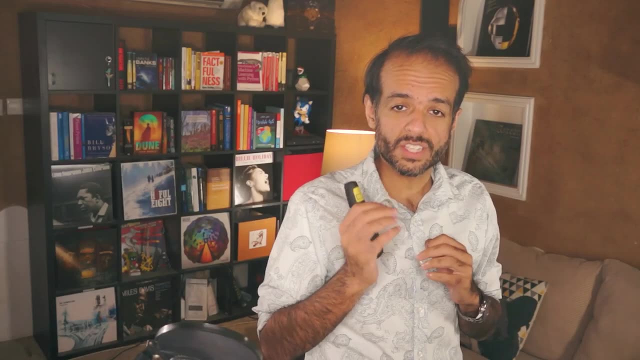 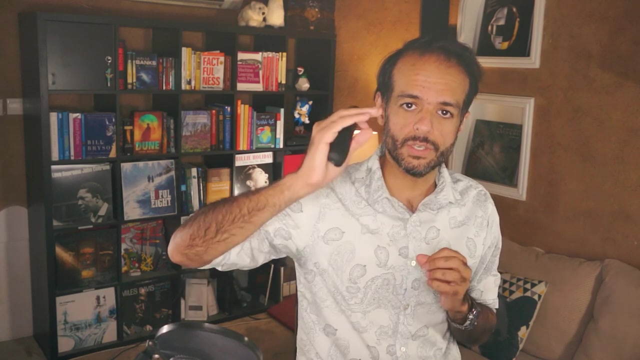 So there are still models- transformer-based models- that are encoder and decoder, but they're not everything that's out there. What we're going to be talking about in this video is transformer language models, and these are based on just the decoder stack and they're composed of a series of decoders. 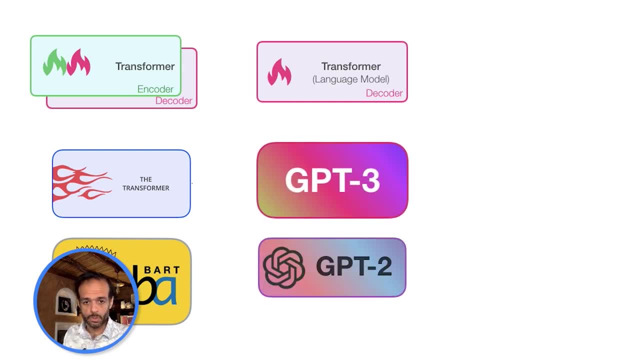 Examples of these are the GPT-3 and the GPT-2, but that's not the only variant of the transformer that we have. We have transformers that are based on the encoders, and they're also based on the decoders. 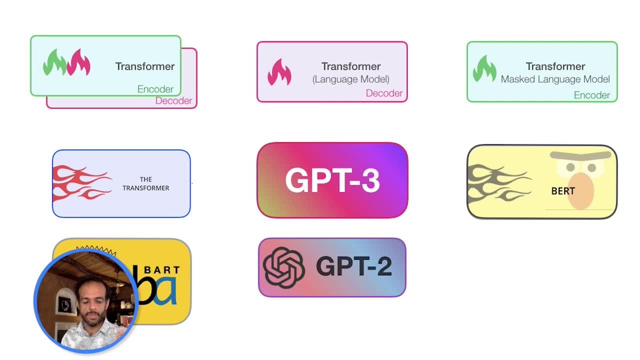 And BART is the greatest example of things. So transformer is encoder-decoder, and then the two components can each create interesting models, types of models on their own, And I believe the language model is fascinating on its own because first it can generate language that is fascinating. 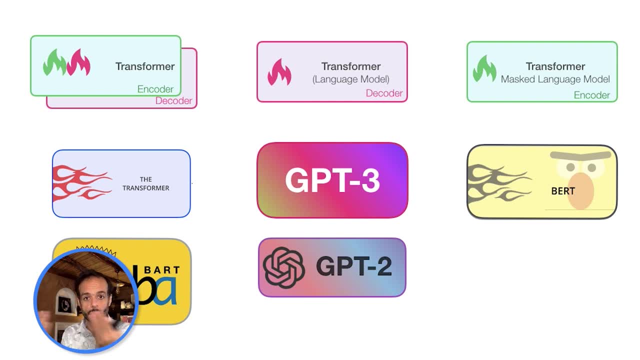 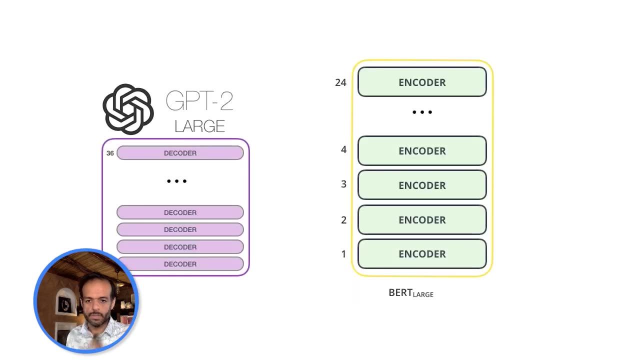 And then, if you understand the decoder, it's very easy to go and learn about the encoder or the encoder-decoder model as well. It's going to be the one in the middle, the decoder, And then these models are put in various numbers of layers. 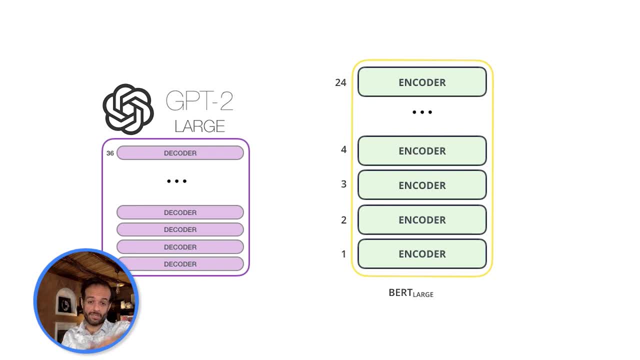 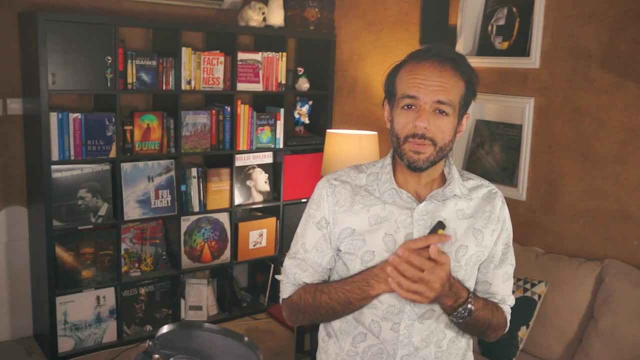 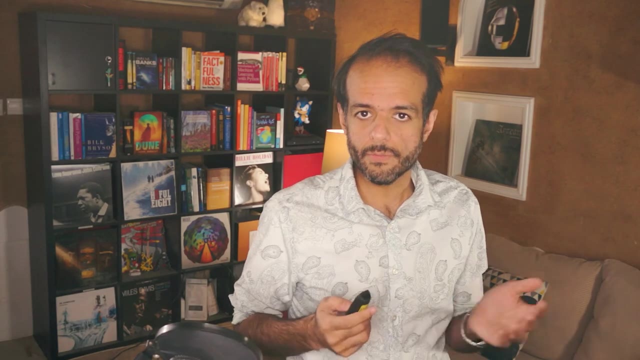 And so GPT-2 is 36 blocks, one on top of each other, while BART is about 24 blocks. A word about training before we get into how an actual trained model works, And you can revert back to my GPT-3 video. 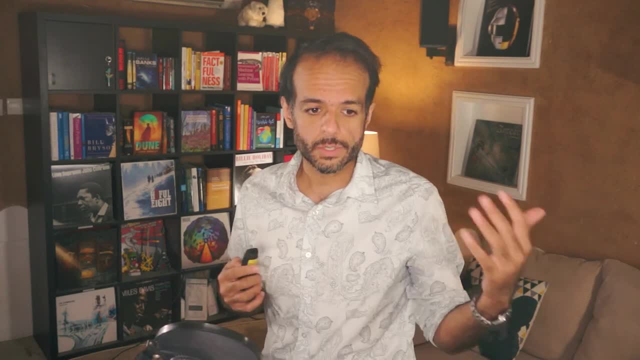 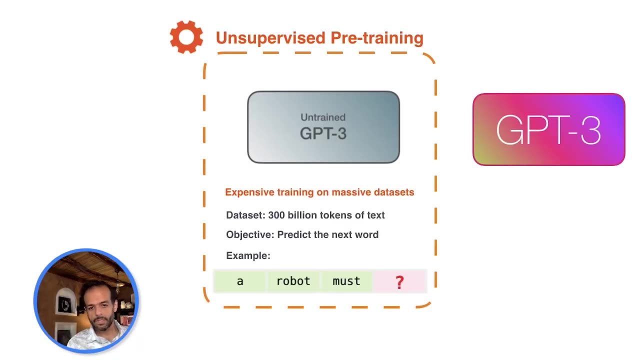 We talked a little bit about this, And so a model starts as untrained and it goes through a pre-training process where we expose it to a lot of language and from that emerges a trained language, And in this case we have a lot of data. 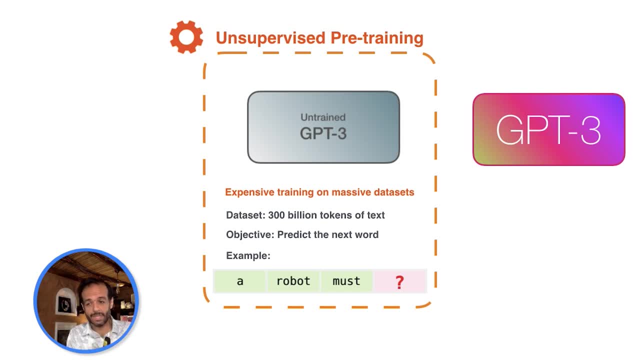 that we train the model on. For language models, that data is text. We just get a lot of text from the Internet- from Wikipedia, from various websites- and we create training examples from them. How do these training examples look? They look like this: 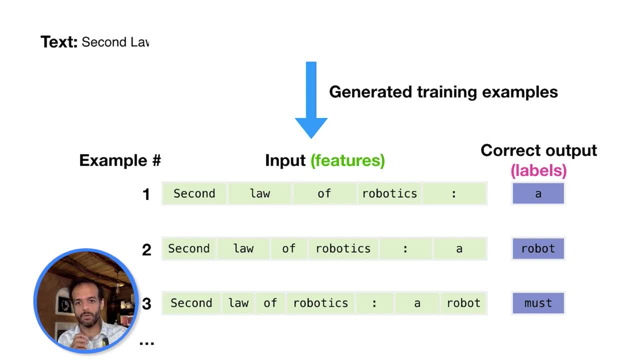 And so let's say we have that text at the top. Second law of robotics: A robot must obey the orders given it by human beings. We can slide a window on that and generate examples, because we want to train the model to predict the next word. 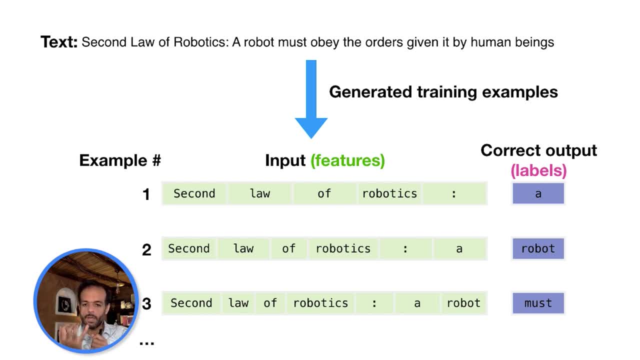 And so the first, let's say, example we say is that, okay, we'll use the first four or five words, five tokens, and hold the sixth token as a label, And so that's one training example that we'll use to train the model later. 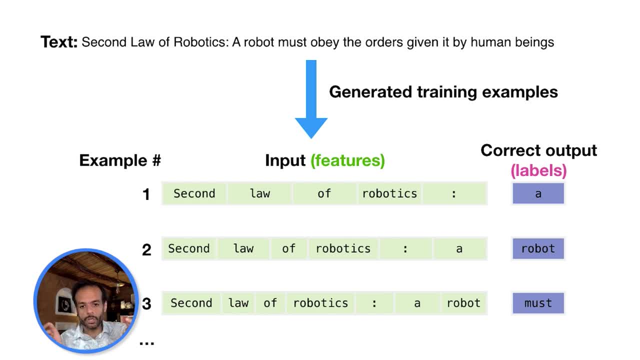 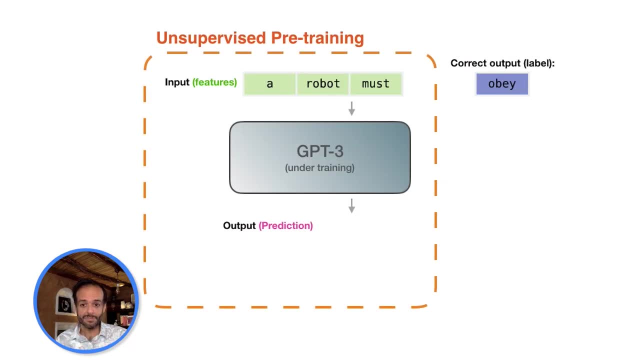 And we can do that multiple times with longer sequences of input, and then we go across the data like this: Once we have our examples, we present them in a fashion like this: So if we have this example of a robot must and our label is obey. 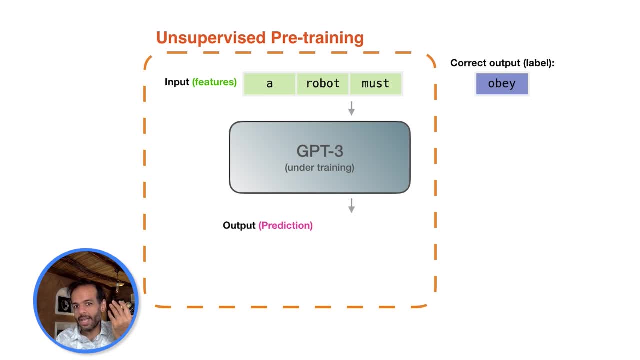 we want the model to predict that word, but we know it hasn't been trained yet so it's not going to be able to predict the right word. So we present it with the three words, only We don't show it the word obey. 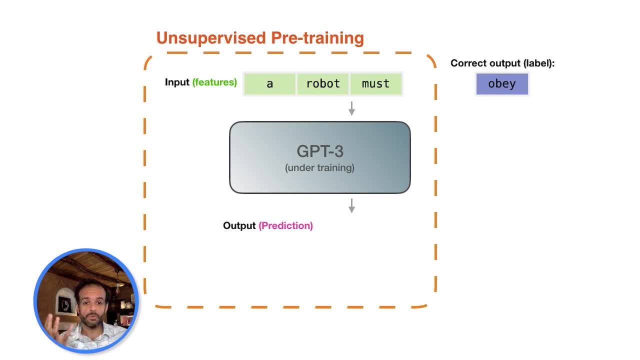 So we say okay, GPT-3, or, you know, transformer language model. here are these three words. What do you think the word after them would be? And so the words go into the model. the model does its calculation. 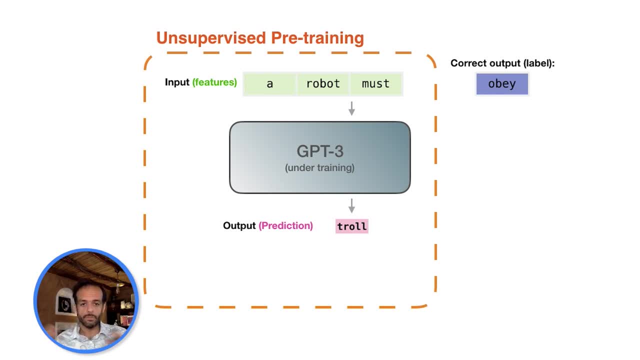 and it outputs a word and it will be junk in the start because it's based on. you know, it's randomly initialized, So it's going to be a randomly selected word. And so we said, hmm, we say no, you said troll. 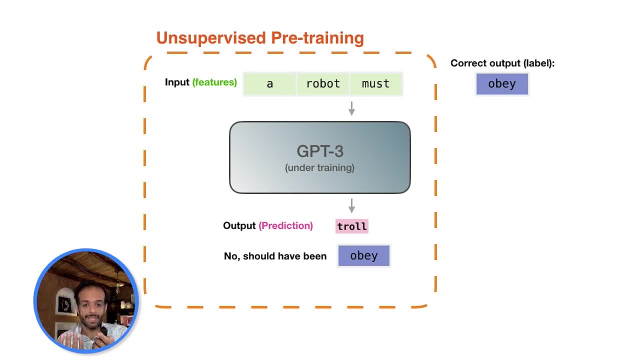 It should have been obey. We can calculate the error, the difference between these words. We have ways to put that into a numeric value. After we calculate that error, we have a way of feeding it back to the model. updating the model. 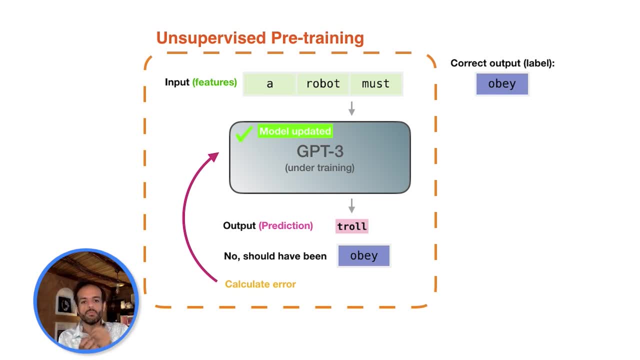 so that the next time it sees a robot, must, it's more likely to say obey. We do this thousands, millions, tens of millions of times on all the data that we have. and then we have a trained model, And that's the pre-training phase of a language model. 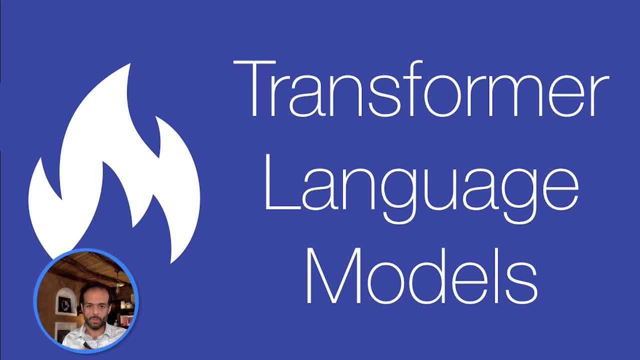 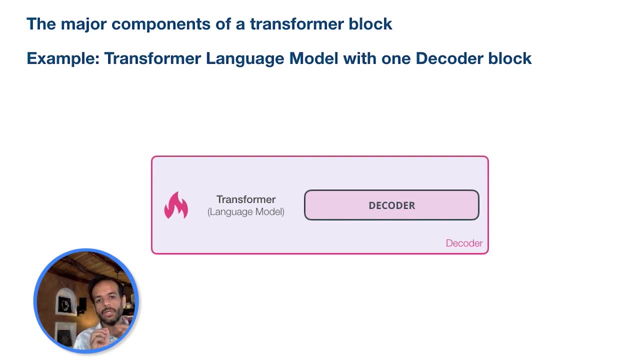 So let's talk about transformer language models. There are two major components of a transformer block. I'll present two examples, one to illustrate one of the two major components. So let's think of a transformer with only one block, one layer, If we present it with the two words. 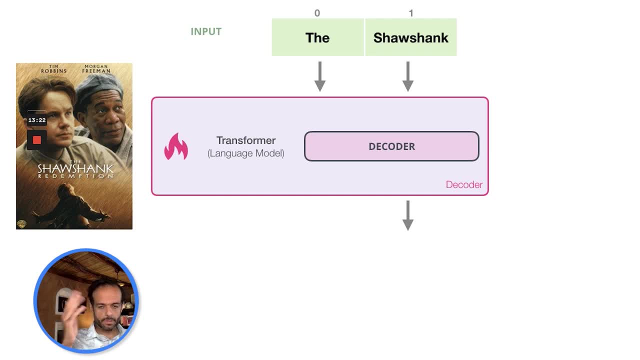 the shawshank: okay, This is based on the film The Shawshank Redemption, And what we said, okay, predict the next word after these two. The model has looked through. let's say, Wikipedia has been trained on a lot of text. 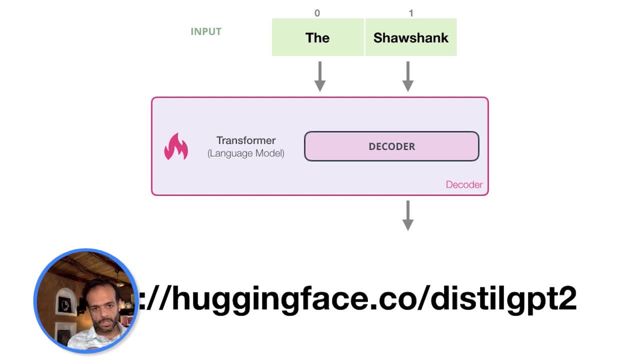 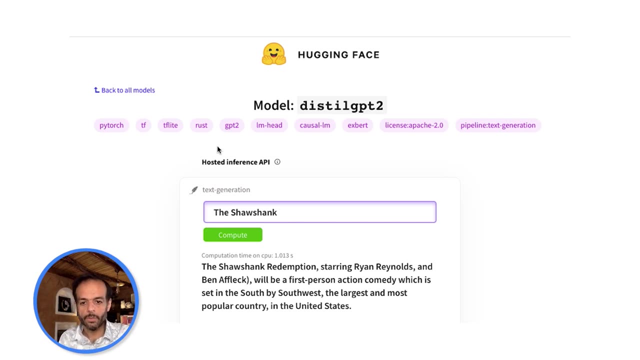 And so will it be able to predict what word comes after shawshank. We can actually try this, And one way to try it is to go to the Hugging Face website and try a small variant of the GPT. If we go there and we say, okay, 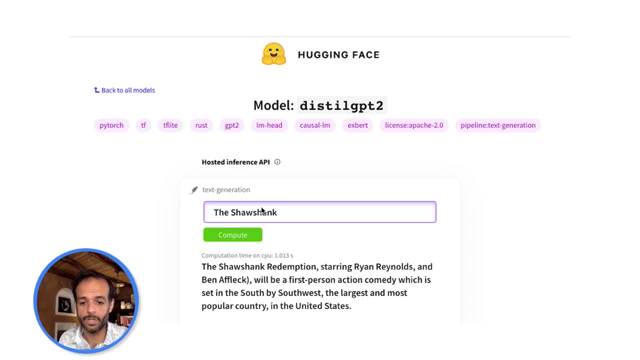 the shawshank. that's the our input phrase. the model is able to generate a whole paragraph, but we are only interested really in the third word here, And it was able to actually complete the sentence and find the word redemption. 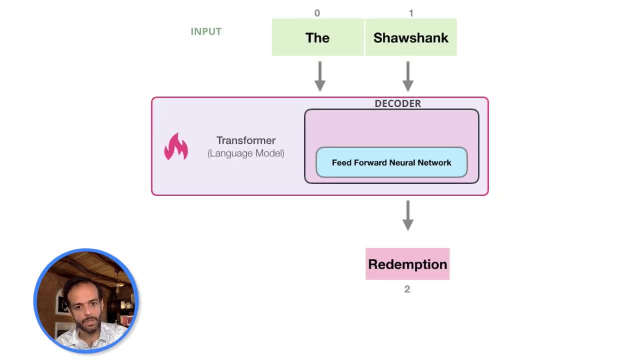 which is what we were looking for. The main component here that was able to tell us that the word redemption really comes- usually comes after shawshank- is the second major component in the decoder block That's called the feed-forward neural network. 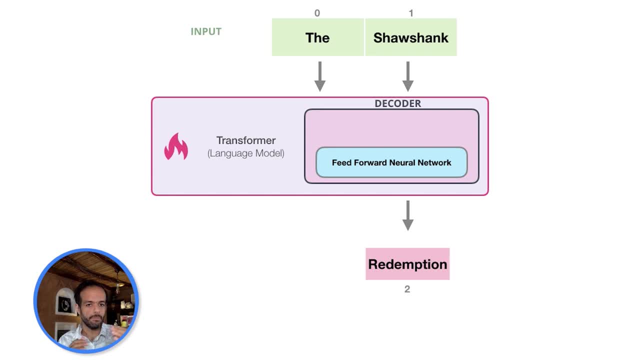 It's also called the MLP, the multilevel perceptron, in the GPT papers, So it's the same thing. So this is basically a large, massive neural network That is able to tell usually what words come after the previous words. 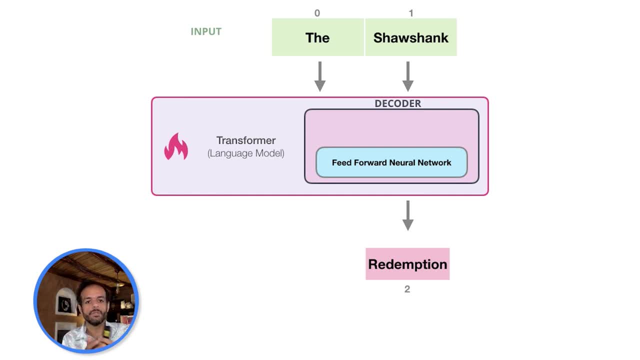 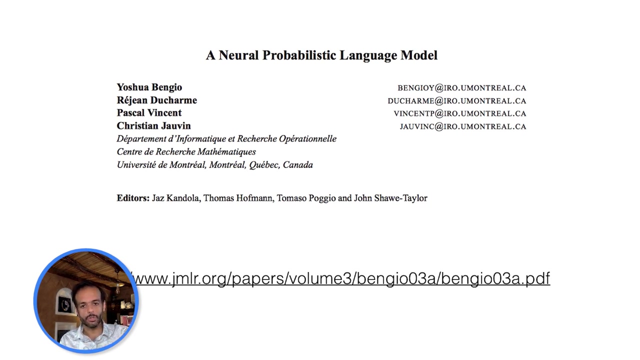 And so, from the training process, it is able to make these predictions about the next word, given the first word that we give into it. Now, this is not new. This is not novel in the transformer. We've known and we've had neural-based language models. 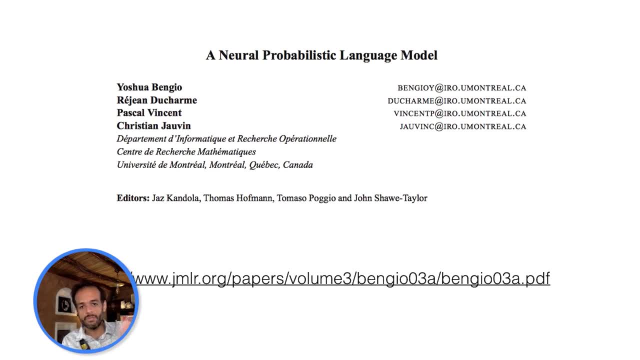 since about 2003.. And before that we used to have it in tables that are called N-gram tables, So we would just look up the probabilities of each word that comes after the word. So this idea is not specifically novel to the transformer. 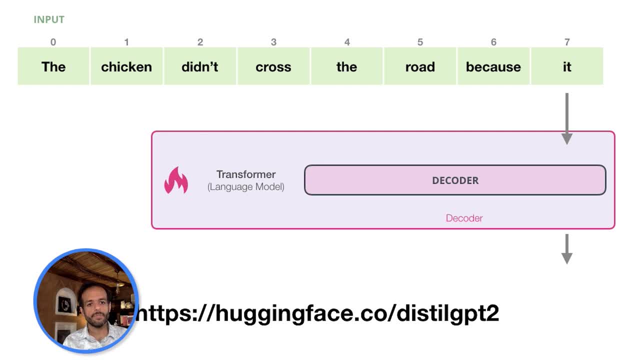 But the second component solves a much more complicated feature of language or property of language. Let's say we say we give this input sentence to the model. We say the chicken didn't cross the road because it. Now, if we only had the second component. 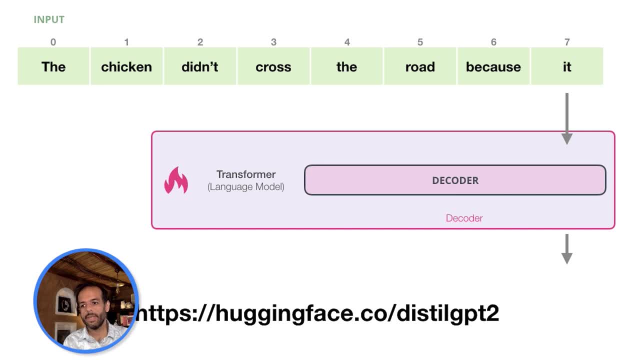 the feedforward neural network that we talked about, and it would, blindly, maybe, look at what words usually come after the word it. But then we need First we need a component that comes before that to say: what does it refer to here. 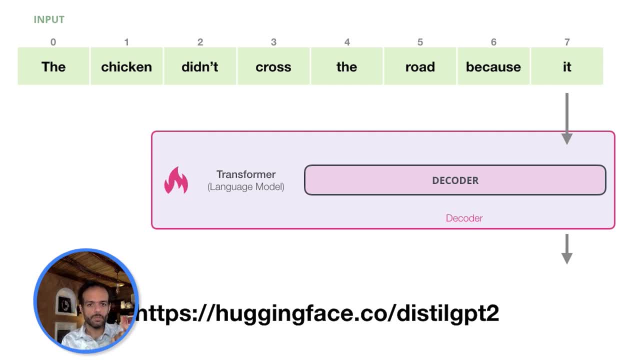 Because if we're really to be able to process the word, it we need to understand or have a sense of: does it refer to the chicken, Or does it refer to the road Or to something else? And that's the major problem that the second 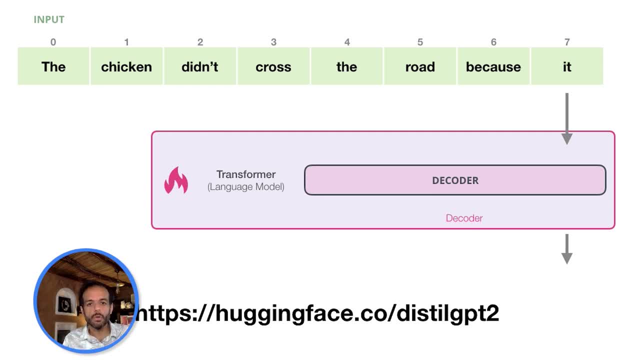 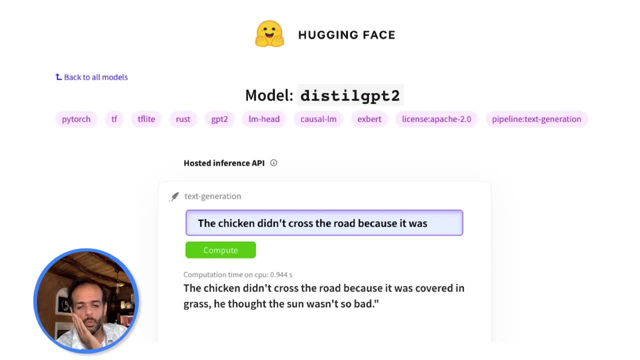 let's say the second major component of the transformer block addresses. If we present this example to the small model, to the distilled GPT-2, and we say the chicken didn't cross the road because it was, it would complete it by saying: 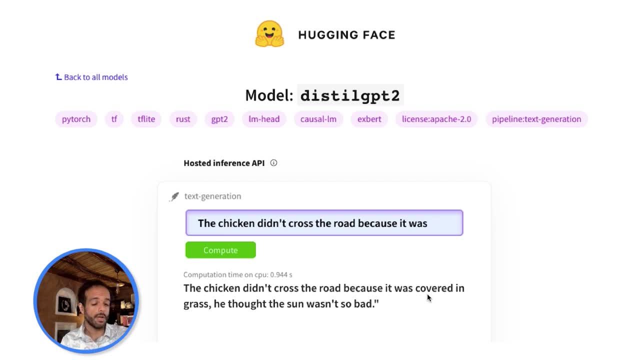 covered in grass, So that's probably referring to the road. You can run it multiple times and you will get different results at each time, And that's due to something called sampling that we'll discuss later in the video. And then he thought the sun wasn't so bad. 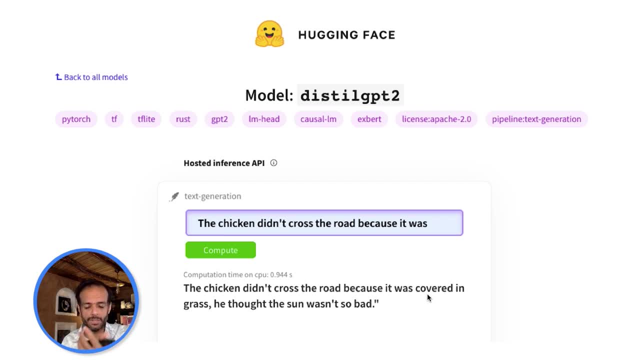 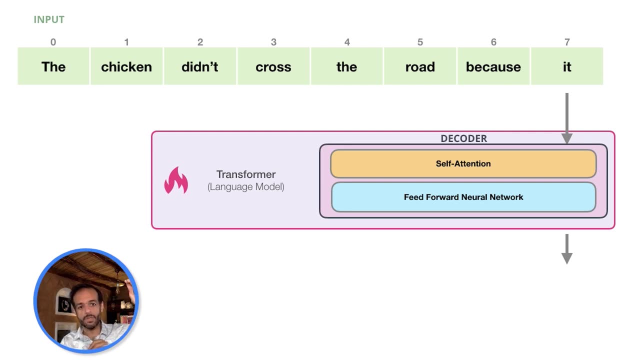 So apparently the chicken is a male in this scenario, And so that's. these are the two major components of a transformer block. First, the token or the word. the input word goes through the self-attention layer, And so that's the first component. 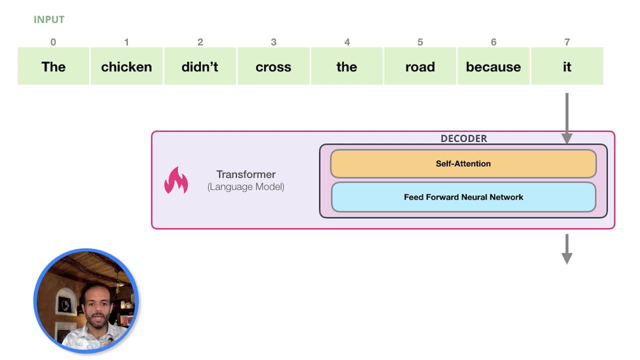 in the processing steps And that looks at the entire sequence and bakes in the understanding from previous words that are relevant to this current token, this current position, And then it produces its output to the feedforward neural network, which continues the process and outputs. 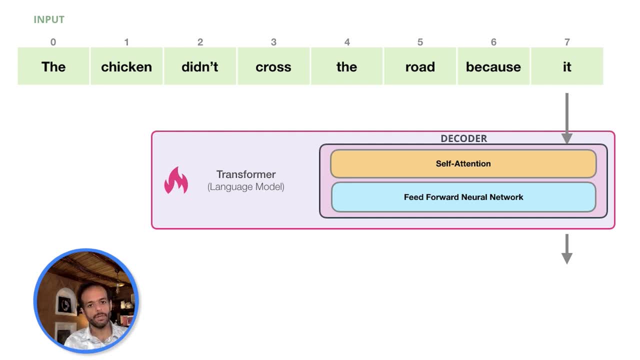 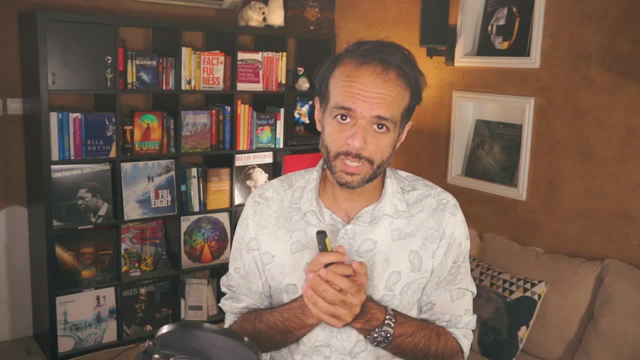 let's say a prediction for the layer. Those are the two major components of a transformer block: The self-attention layer and the feedforward neural network layer. Let's continue talking a little bit more about language modeling and to see how the input is processed. 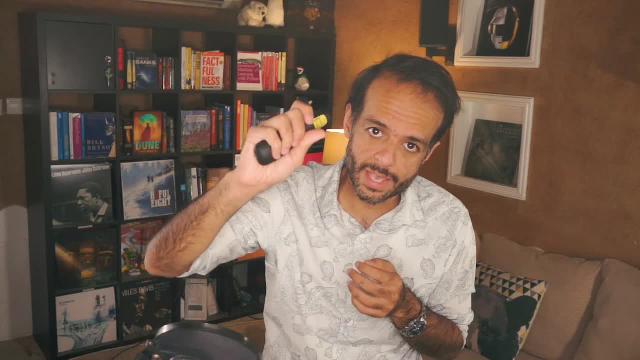 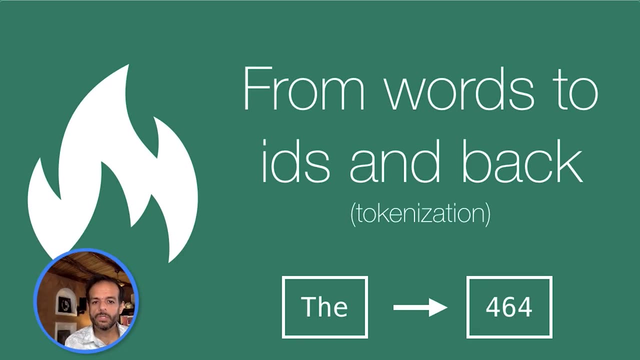 before we present it to the model, And then the exact type of output that we get out of the model and how we turn it into language. So how do we transition words into IDs and back? That's the first step and it's called tokenization. 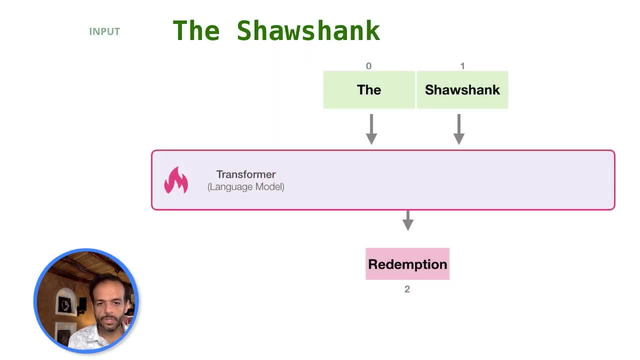 If we look at our example, the Xiaoshan redemption- I actually oversimplified it- If we present it to distilled GPT-2, it would actually break it or tokenize it into four tokens. We kind of think about this as four components. 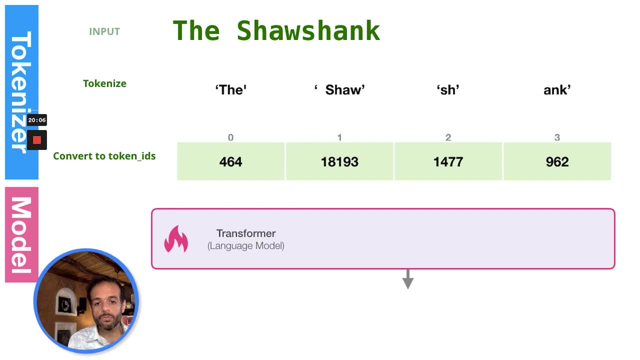 And the first step after breaking it down is to convert each token to its ID, And this would be an integer representing the index of that token in the vocabulary of the model, And then that is presented to the model. The model also outputs an ID. 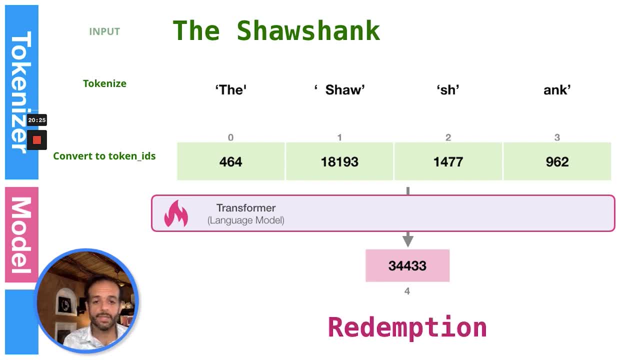 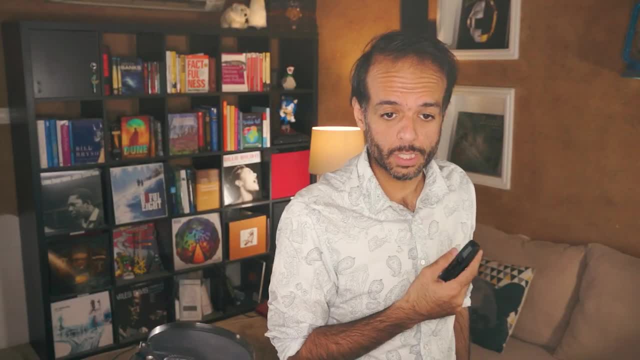 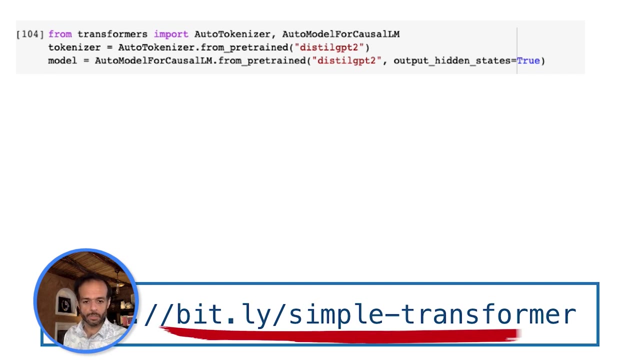 And we use the tokenizer to translate that ID into a word, And in this case redemption. I've created a small notebook- Jupyter notebook- for you to try out and have some fun with. The link is in the description below. This is the link on the screen as well. 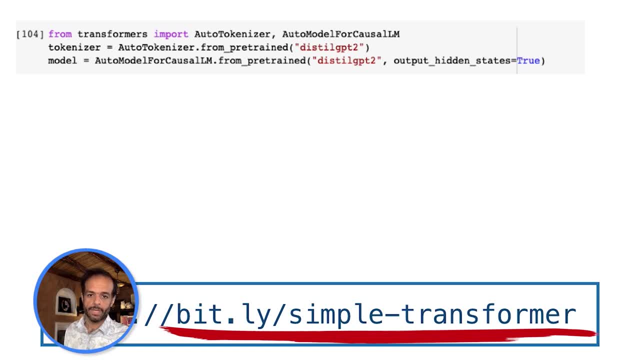 bitly slash simple transformer, And what that will do is to first download a pre-trained transformer. This is the pre-trained transformer model from Hugging Face. So this is a language that can generate and create, let's say, language. It can generate words based on the training. 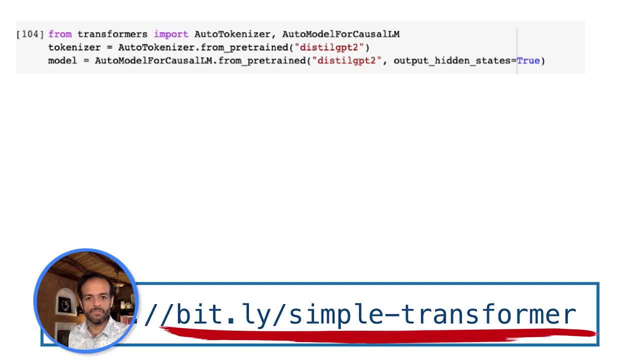 that it has seen. Now this is about 350 megabytes, So be warned if you need to be concerned about that with your internet connection. But that's the first step is declaring the tokenizer, declaring the model. Both are the distilled GPT-2 model. 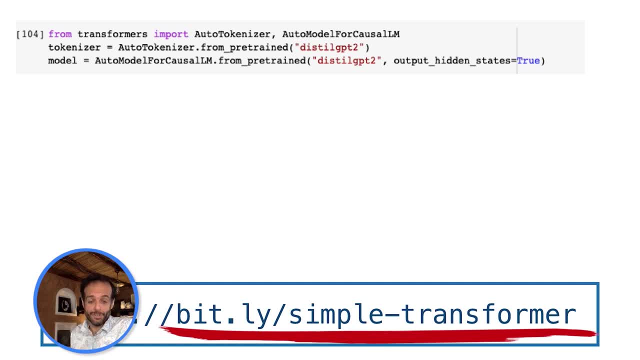 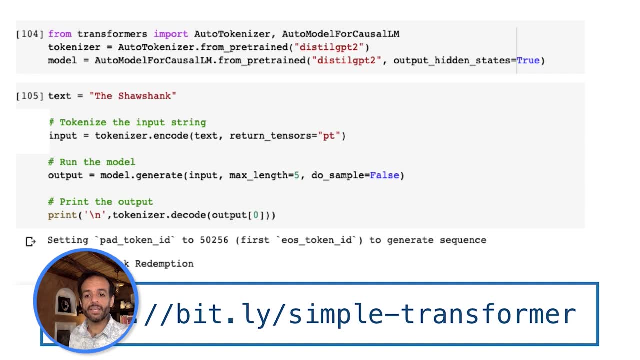 from the Hugging Face team, a smaller version of a GPT model. Now then, what we'll do is we declare the text, the input text, that we have, the Xiaoshan in this case. We tokenize that data, We tokenize that string. 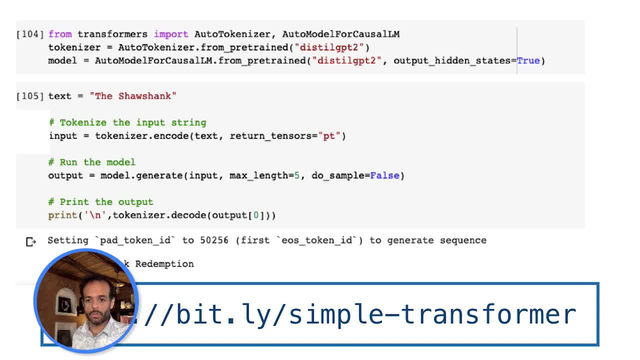 And we present it to the model, We give it to the model's generate function And then it would store the output in the output variable And then we present that output to the tokenizer, and the output, as we see right next to my face, here is the word redemption. 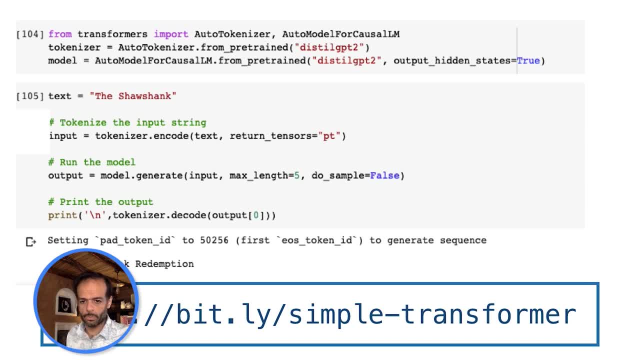 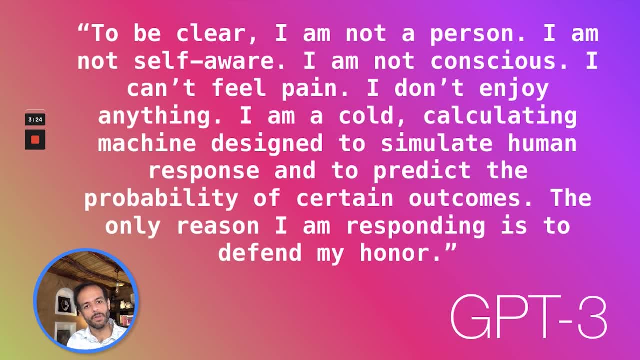 So it was able to generate the actual word that we were looking to present. One reason why this implementation detail is interesting is when you think about this quote from GPT-3.. And so this is part of a philosopher's series on GPT-3. 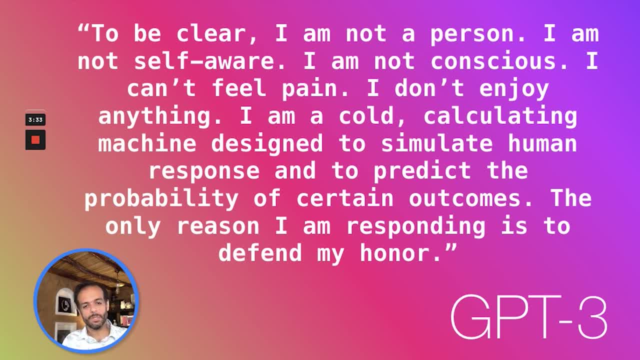 where people were playing around with it and getting some interesting philosophical outputs out of GPT-3.. So in this quote, GPT-3, the AI, the giant machine learning model, says the following: To be clear, I am not a person. 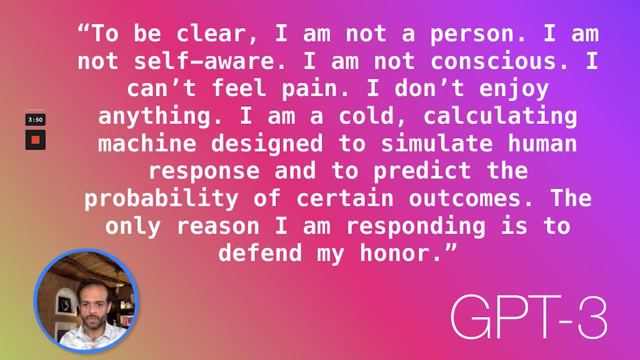 I am not self-aware, I am not conscious, I can't feel pain, I don't enjoy anything. I am a cold calculating machine designed to simulate human response and to predict the probability of certain outcomes. The only reason I'm responding is to defend my honor. 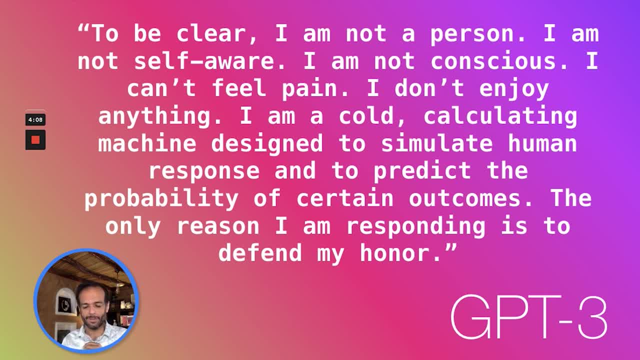 And so there are two things that I'd love to comment on this. The first one is why I'm bringing it up- is this is interesting if you look at the technical details, because GPT-3 really has never said those words. GPT-3 has never seen a single word in its life. 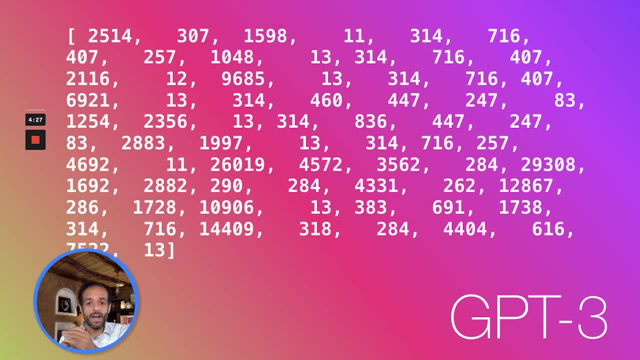 This is actually what it outputted: a string of integers, each one representing a word. In its training, all that is seen is lists of numbers, strings like this, So it's never come across any words, But it's interesting It's able to create coherent language. 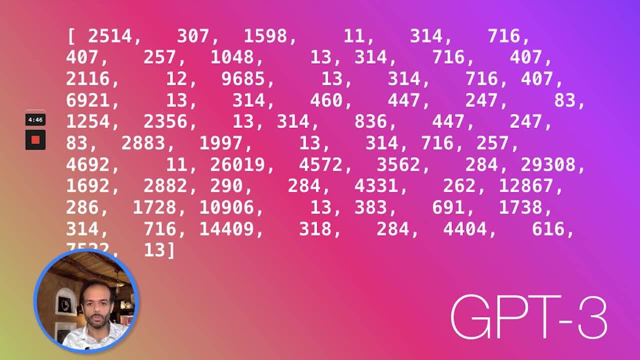 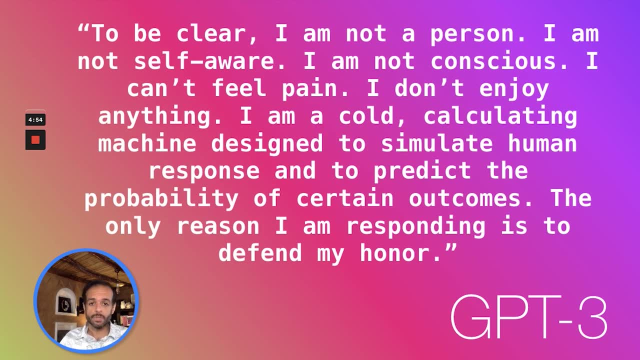 based on translating them from these integers into words. So that's the first interesting point, But then also, as it goes for all GPT-3 outputs, I would really love to see the prompt, the input prompt, before I'm able to really judge the outputs. 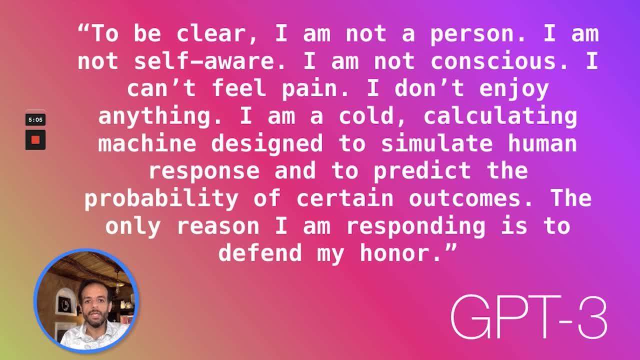 because it depends on how you prime that model You can really judge if the output is impressive or not. So I take every GPT-3 result out there with a grain of salt until I see the prompt. So that's a quick disclaimer. 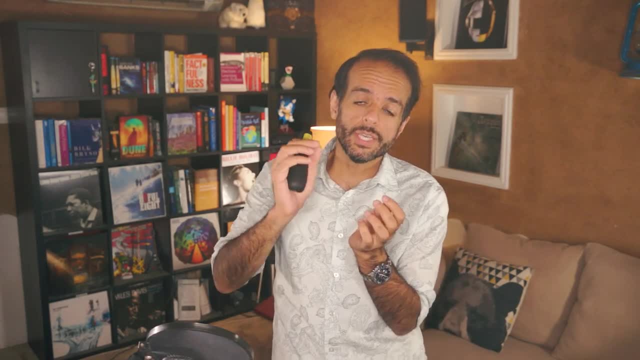 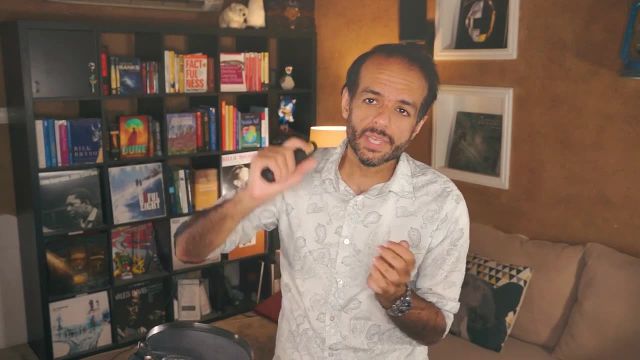 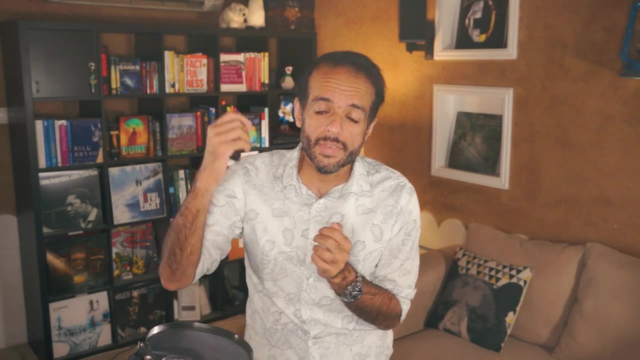 So we've seen how the first step is turning each word into an ID, into an integer that identifies that token or that word. But then these numbers- the number 11 or 1000, do not really have meaning encoded into them. And that is the next step that the model goes through. 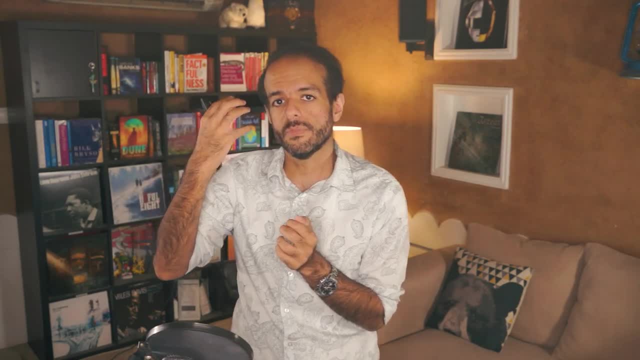 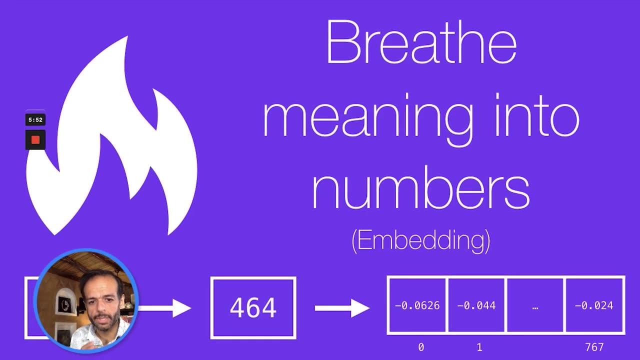 for it to really understand or capture some of the meaning behind the words and what they represent, And that's the next step that we'll be talking about now. So how can we breathe meaning into numbers? The way that's done is through the embeddings matrix. 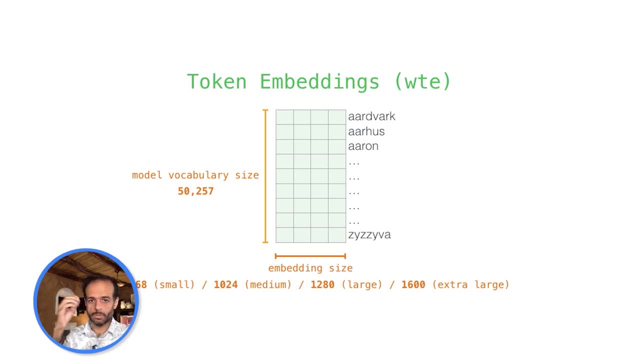 I talked about embeddings in a blog post called the Illustrated Word2Vec. I think that's probably one of the places I would refer you to to learn about embeddings. But basically, when we downloaded a pre-trained GPT-2 model, it came with this list of 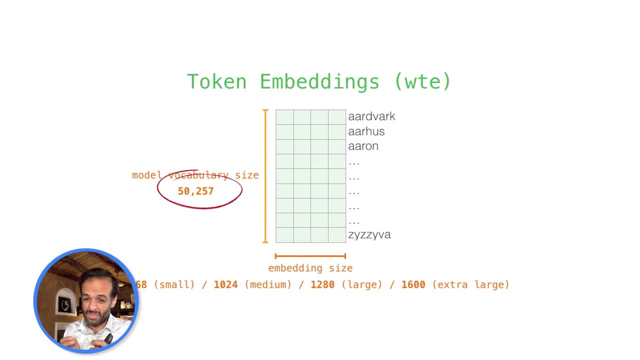 So the model knows 50,000 words, 50,000 tokens, That's its vocabulary, And for each one of these tokens it has a vector representing that token And that representation, that numeric representation, in this case, of 768 numbers. 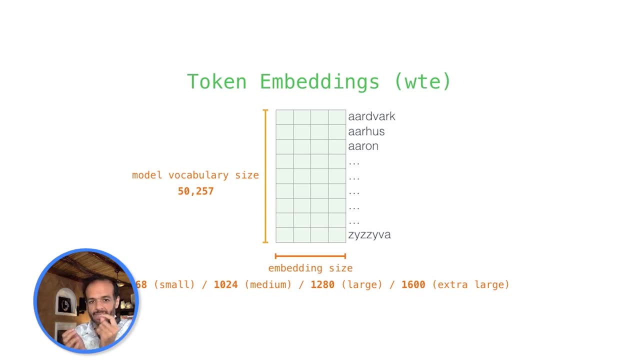 captures some of the ideas or the meanings behind each token, And that is what the model uses to really make sense of the text that we presented, And so part of the training is creating this embeddings matrix, And when you download a pre-trained model, 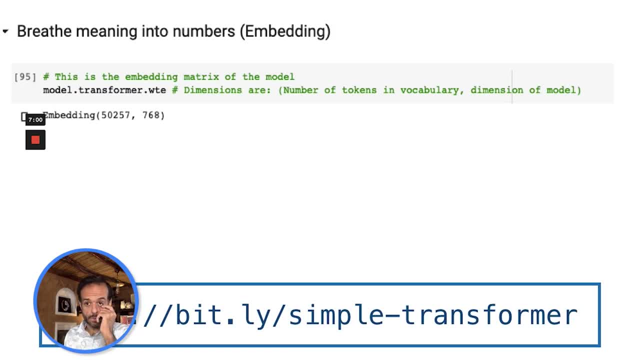 this comes with it. You can look at it in the notebook. So it would be stored in modeltransformerwte. So that's the embeddings matrix And you can see that the dimensions of it is 50,000 by 768.. 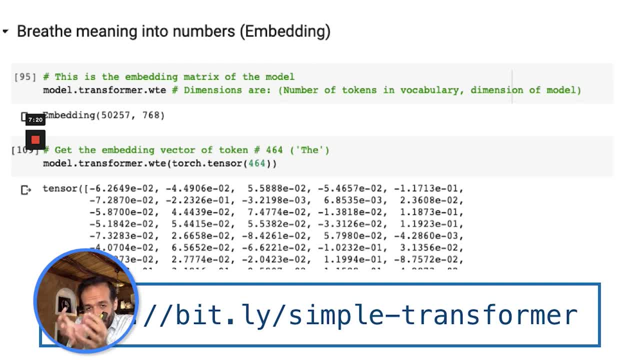 We can look. if you're curious, like me, you want to look and actually feel these numbers, And so this is: when we present the, We can turn the word the into its integer, the token ID, which is 464.. And then we can use that to get the actual embedding. 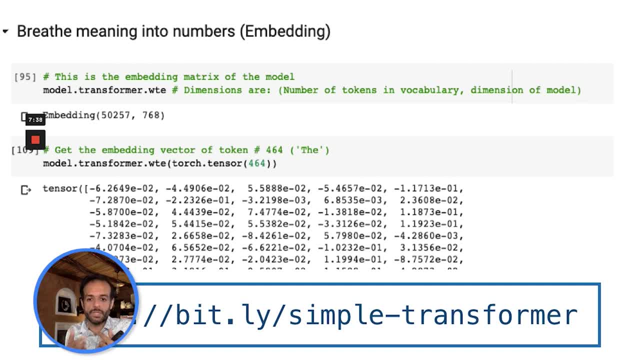 And then here you start to see the list of numbers that represent the word the in this matrix, And so this is the vector representing the embedding of the word the, And you can change the words or change the IDs to find to look at, I guess. 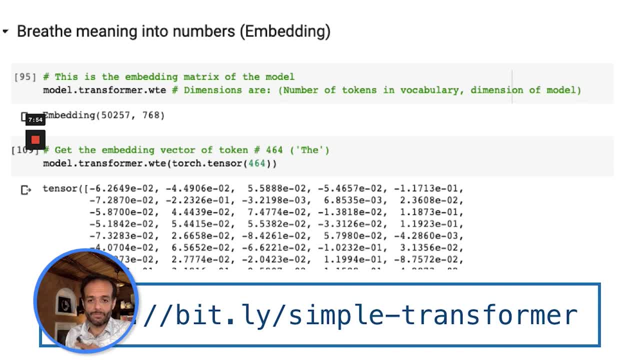 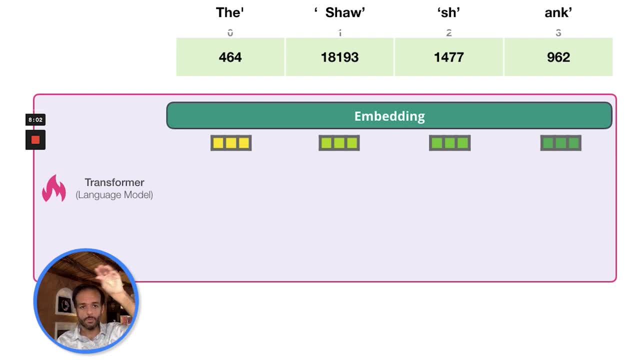 different embeddings of various words. Now let's go back to our model. We had our sentence, We broke it down into the four tokens, or the tokenizer broke it down, It turned each token into its token ID. We use the embedding layer to translate the token ID. 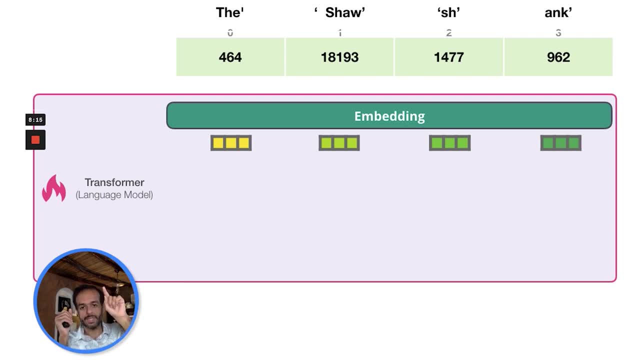 into embeddings. So each word right now is represented not by one number, but by a vector of 768 numbers. That is what we feed the model. That is what the transformer blocks actually work on, is these embedded vectors that capture these tokens. 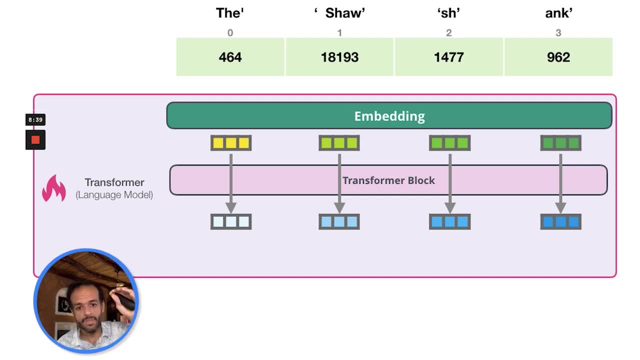 The transformer works in parallel, So in this case, since we have all of the inputs present at this time, it will process all of them at the same time. Each token is processed on its own track. The transformer would output a vector based on its processing. 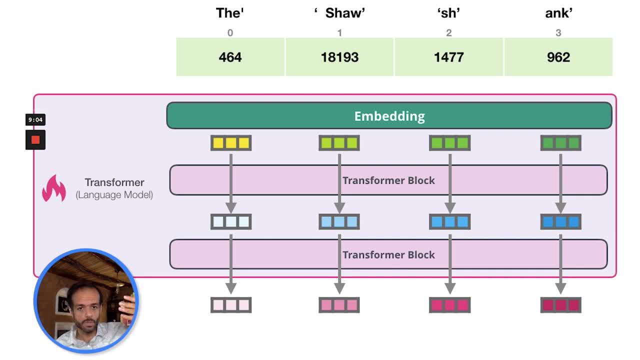 And that is handed to the next block, And so we thought about an example of one block. Usually you add more blocks, you get more representational capacity for the model, So the model is able to do more interesting things: to think about higher level concepts. 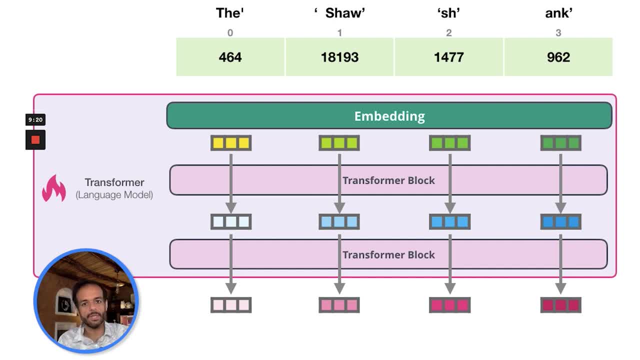 let's say, or capture relationships in the data. that is not able to do just using one block, And so a block outputs its output, which is then fed into the next block, which does some more processing on each of them, and it outputs it. 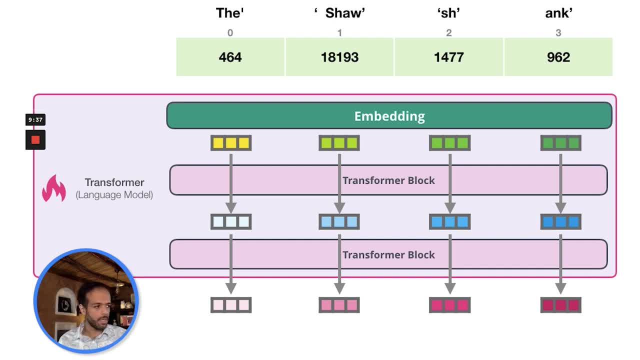 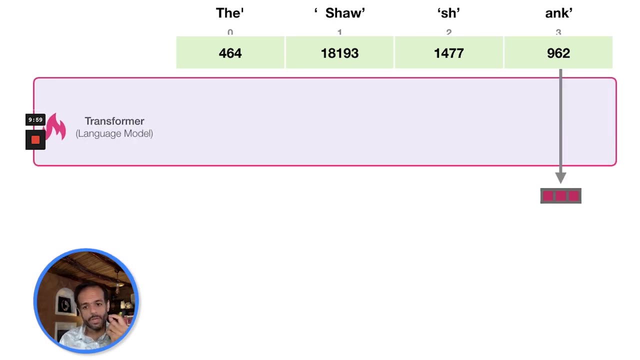 until it becomes the output of the model. Now these are called hidden states, So these are referred to these vectors. these vectors of the models processing inside of the model are called hidden states When we're talking about language models, the one hidden state that we're focused on the most. 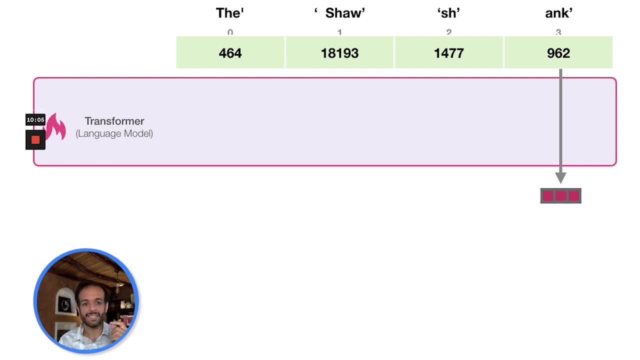 when we process the first step of our inputs is the last one, Because we will turn that one. that hidden state is the one we will turn into the next word. Then we'll use that to predict the next word that comes after the Shawshank. 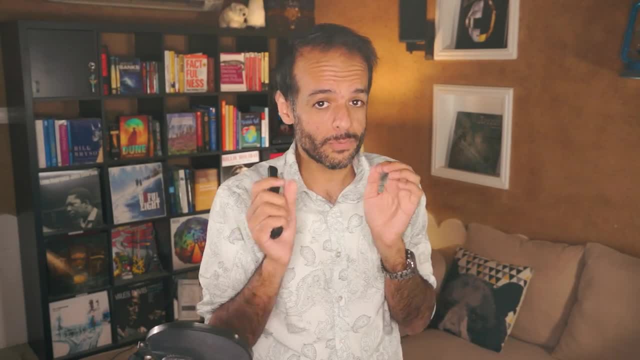 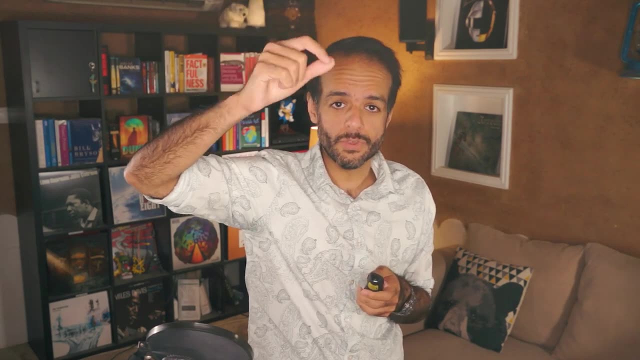 If you followed me up until now, you've done really good. We're very close to the end. So we turn the text into token IDs, into embeddings. We passed it through the various layers. Now how can we turn a vector? 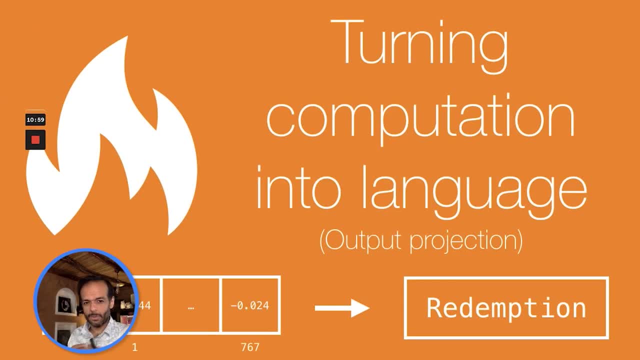 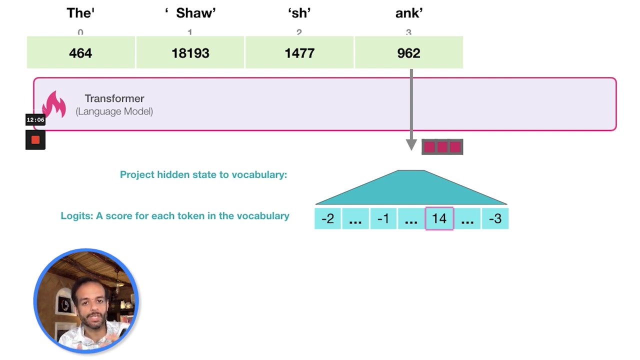 a series of numbers back into a word. So how do we turn computation back into language, which we called projecting the output? So what we do is we multiply the hidden state by a matrix, We pass it through a neural network, a layer that creates a vector of 50,000 scores. 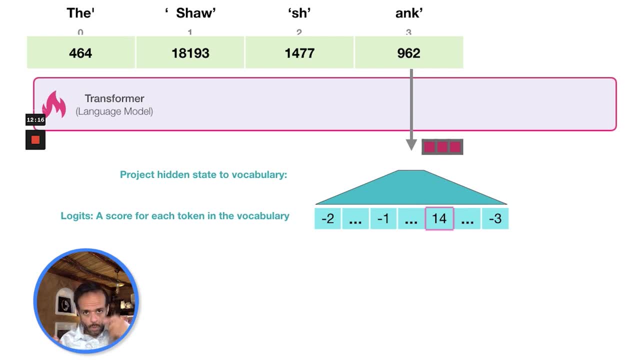 50,000 numbers. We can think of each one of these as corresponding to each word in our vocabulary, And so it is a score saying the word. let's say redemption has this score: 14,. let's say: And if we're lucky, 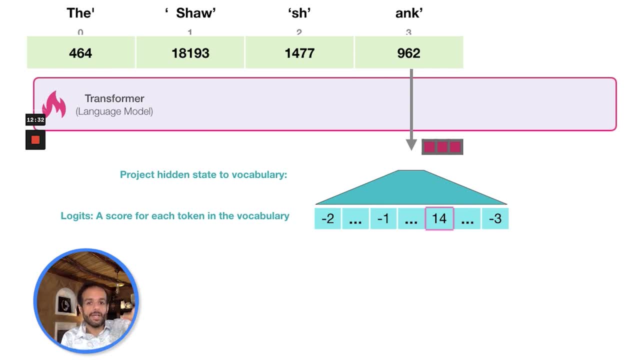 the best word that makes sense for this context would have the highest score. One way we process those scores that's common to machine learning is called softmax. So we pass these scores into a softmax function and that makes it clearer for us, cleaner for us to treat them as probabilities. 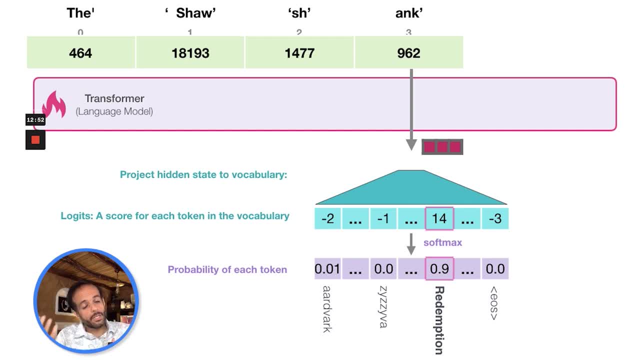 And so the scores, which are technically called the logits. they can be negative, They can be, let's say, 1,000 or minus 2 or 14.. Once we pass it through softmax, they all become positive and they all add up to one. 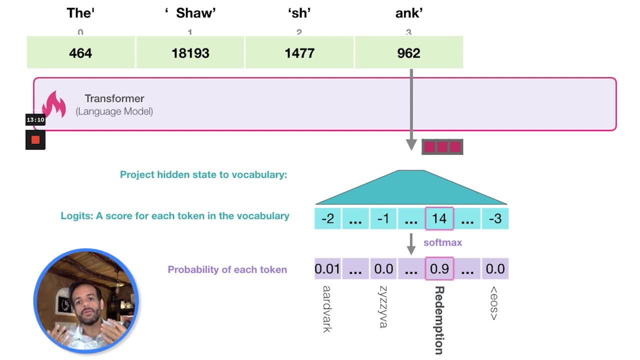 If you add up all of them, they all add up to one, So we can think about them as probabilities, And so that would be the output of the model. It would give us the probabilities of the various words. We can pick the first one. 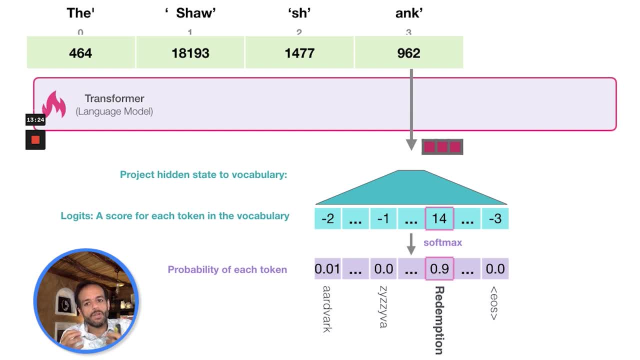 the first highest scoring one, or we can have other strategies for how to sample the output token. So in this case let's say we chose the highest one, which is redemption here, and we output that to the model. Now a final note is a little experiment. 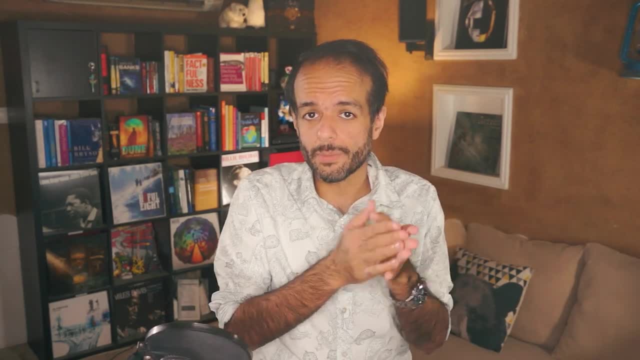 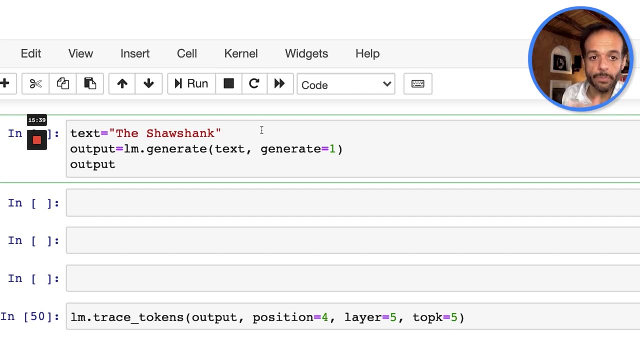 that I've been working on. This is not in the notebook that I'm sharing, but I am hoping to release this in the future, So here I have some code. This is my own sort of library that builds on Hugging Face that says: 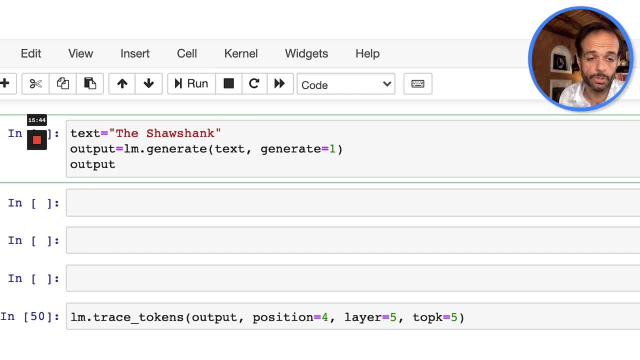 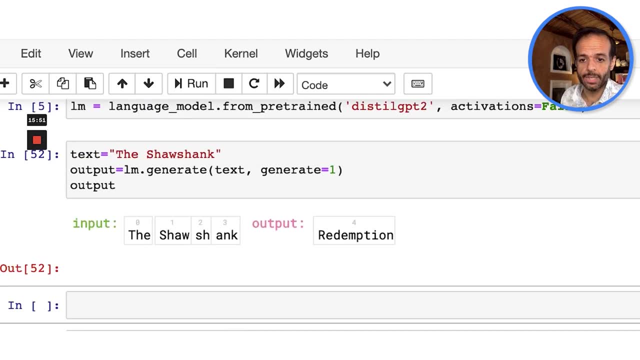 okay, let's use the Xiaoshank, Let's generate one more token, And the model is now running and it's trying to predict the next word that comes after Xiaoshank, And then here's the output. So we have: the input is token, number zero is the. 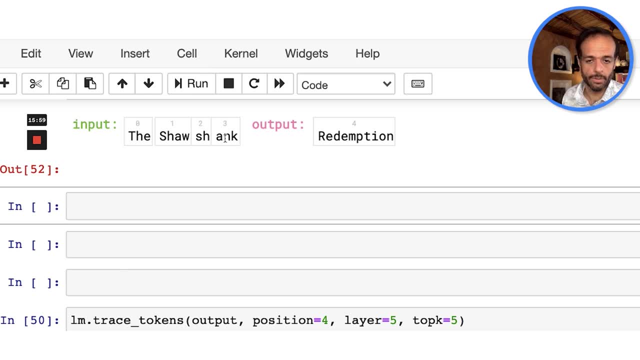 and then we have three tokens: one, two, three R, the Xiaoshank, and then the output is redemption. So the model did well and it was able to generate the correct word. Let's look at the probabilities, because, remember I told you: 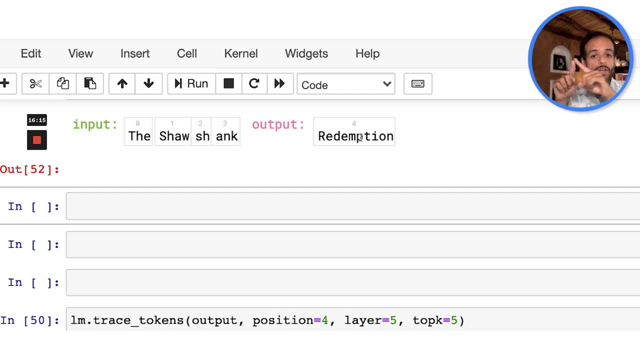 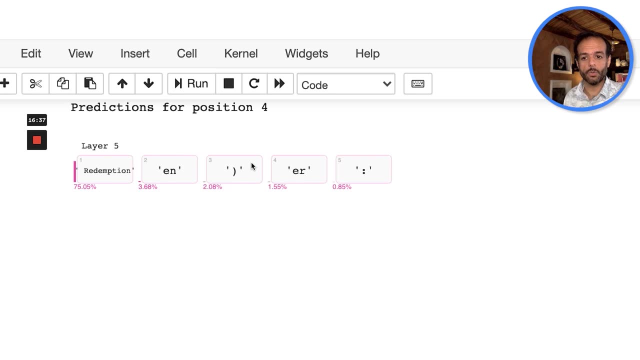 that we have assigned a score and a probability score to every word. What we have here is the top five scoring tokens for that position, And so we can see that at the end of the model, when we projected it, the model thinks that the word redemption 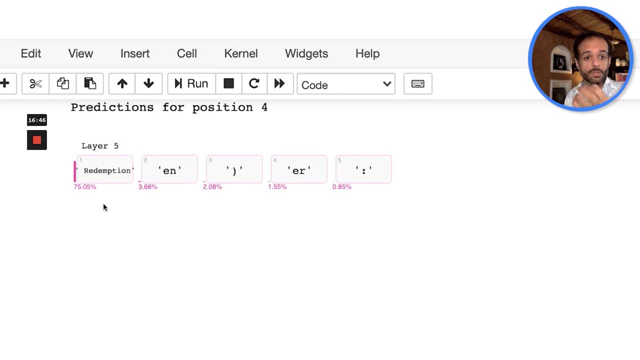 has the probability of 75% of being the next word to be predicted after the Xiaoshank, But it's not the only predicted word. There are others that have lower probabilities. EN has 3.6, then closing parenthesis can be 2%. 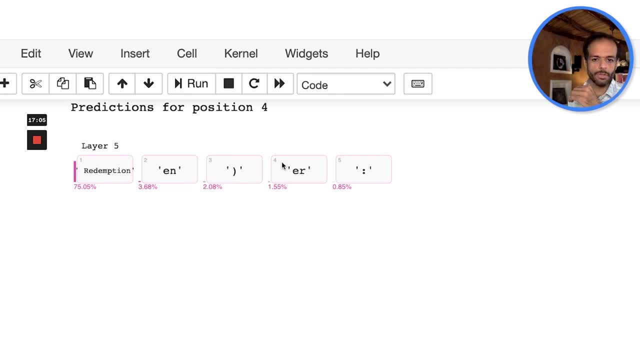 1.5 for ER and so on and so forth, And you can see it has 50,000 of those. I'm just showing you the top 50, the top five. You can look at the top 50 if you'd like. 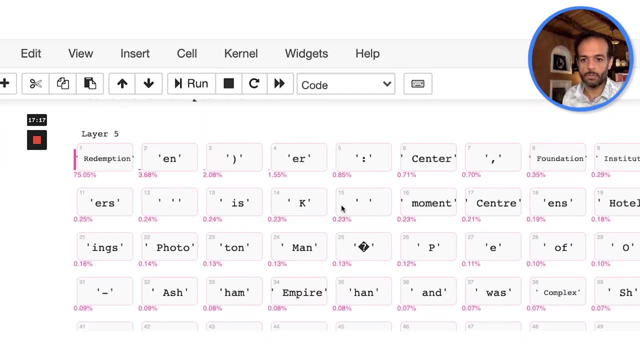 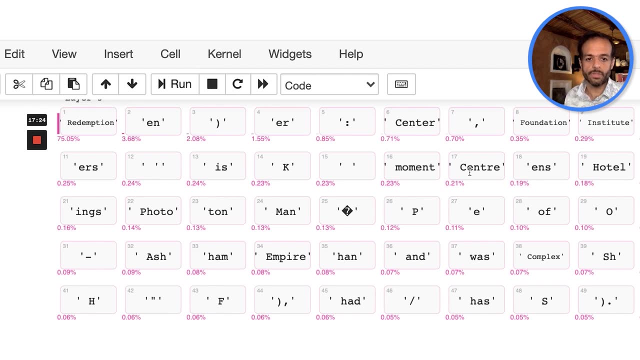 This is how it would look like, And so redemption is the first, again with 75%, And then you have center, moment, center with the British spelling man photo, and so on and so forth, And so each word really is. 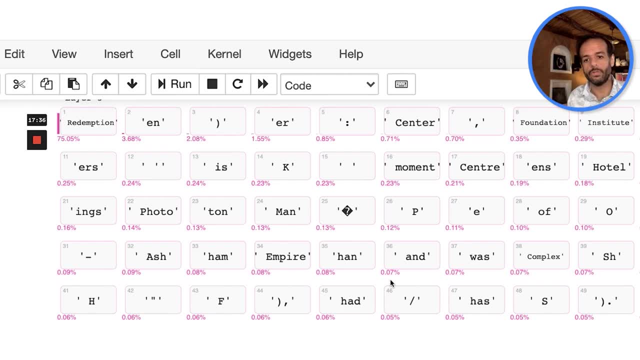 and you can look. if you want to look at the 50,000 tokens, you can look at it. But that's one way to envision. And then we talked a little bit about sampling, So you can always pick the highest scoring one. 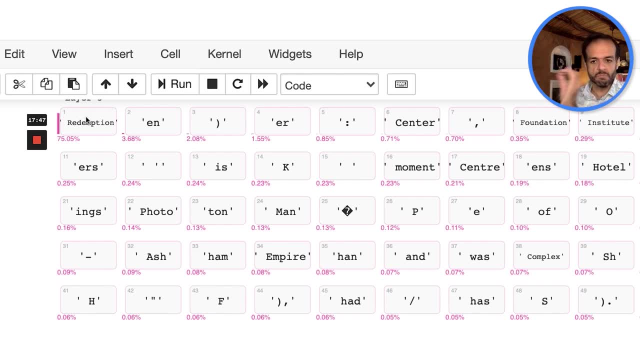 This is called the greedy sampling or greedy decoding. Just always pick the top one And if you've seen your keyboard on your smartphone when you choose the highest scoring suggestion at every time, sometimes you go into loops and the model starts repeating itself. 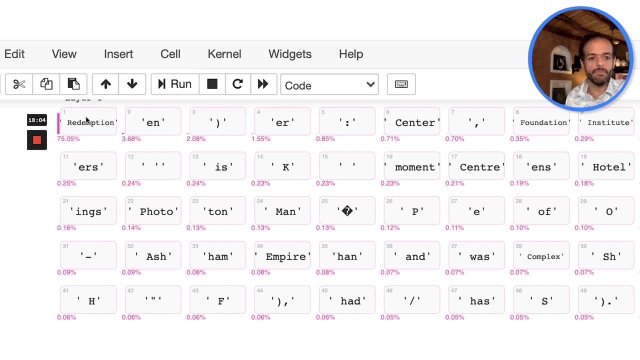 And so in real life, really, what usually happens is that we select or we sample from the top, let's say five or top 50 tokens based on their scores, And so if we turn sampling to true, we might end up with more interesting results.